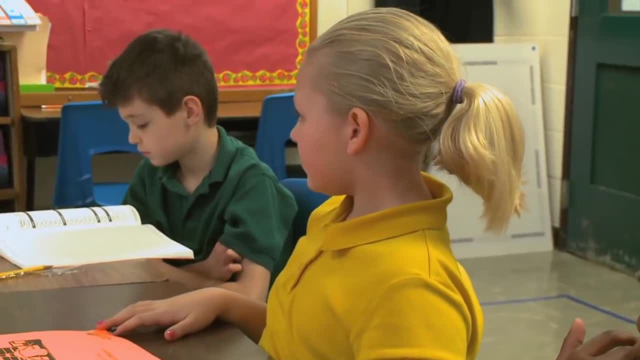 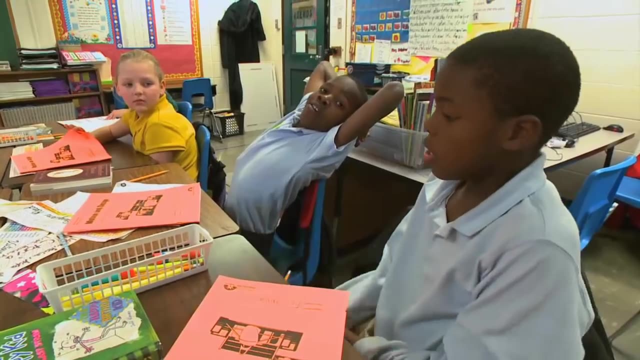 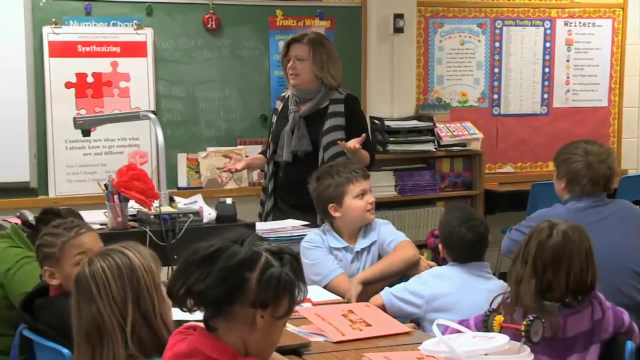 Motion is a change of position. Motion is a change of position, And to change a position, you need a what? A what? Jackson? You need a force. Forty-万. yes, You need a force, good job, good job. And what can cause that force? 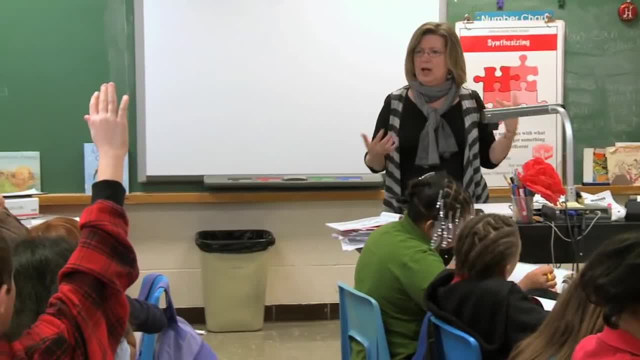 I know we've made some vehicles and we've made the move. What causes that force? None. What causes a spell? Ah, Isaiah, Um, All right, you've moved it a little bit, любِعَفْضِعَ. 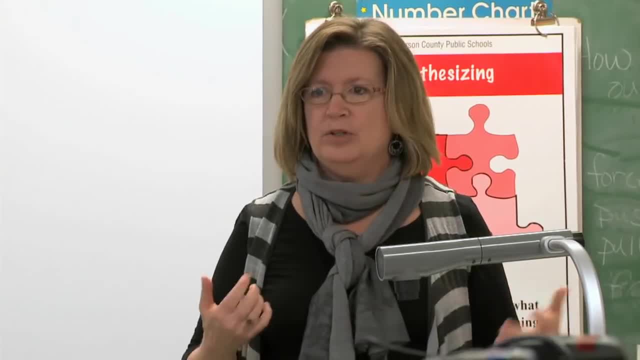 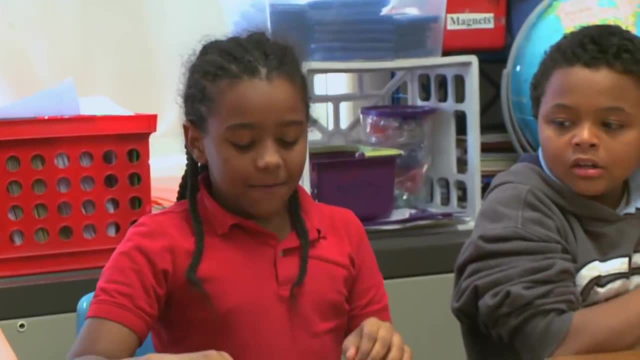 I can A pushing or a pull, A push or a pull. Okay, How do we provide that push or pull that gets our vehicle going, Ramona, Like we can push in and like, say this, the vehicle, we can push it and it start rolling and 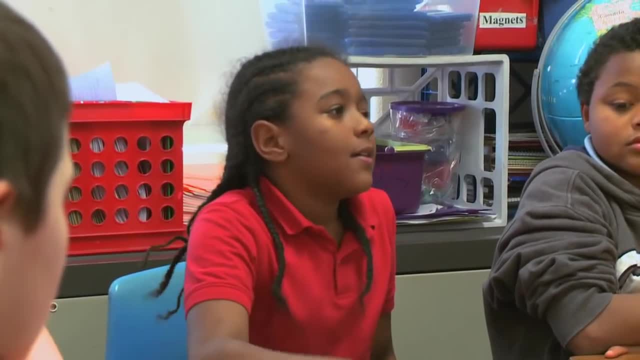 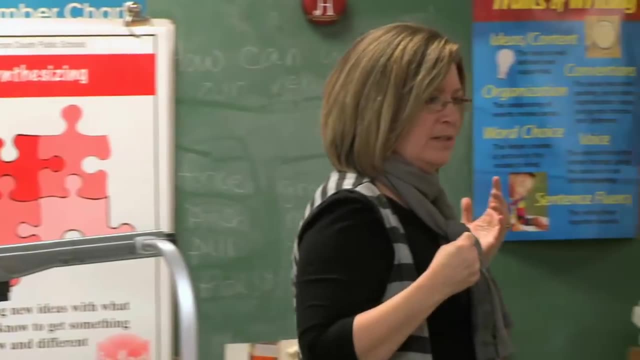 Assume that you need pressure to pull. yes, everything changes. So you can use, Use your hand, your own force of your muscles. Good, How else can we get this to move? What's on your mind, Preston? Anything? 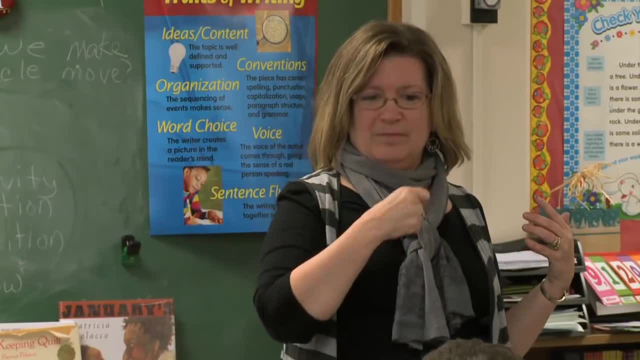 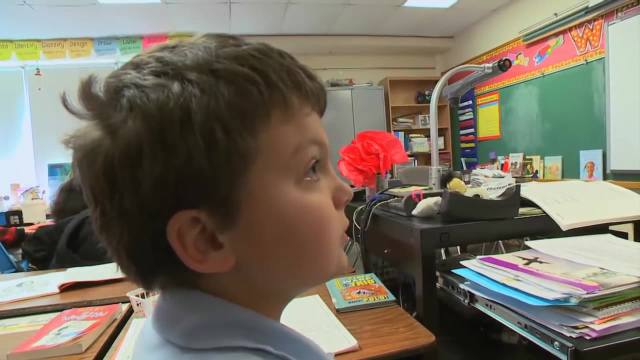 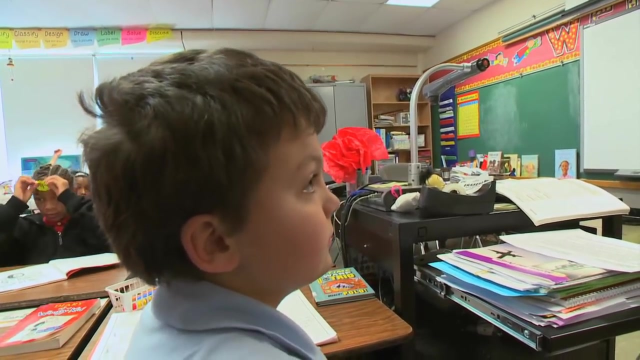 No, Okay, We can blow on it and it will. Okay, so what does that do? Good, We can wind, and wind does what? Push It, pushes it, Good. good, Any other ideas? You can touch it with your hand and start pushing it forward. 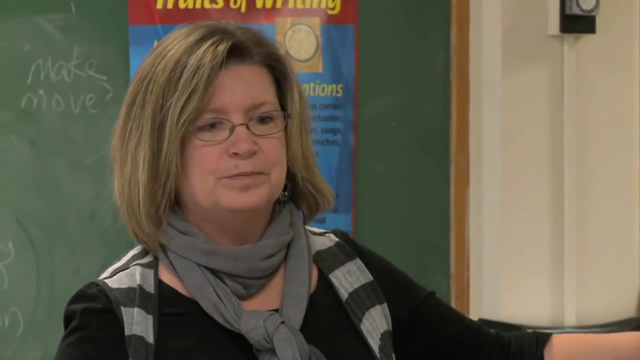 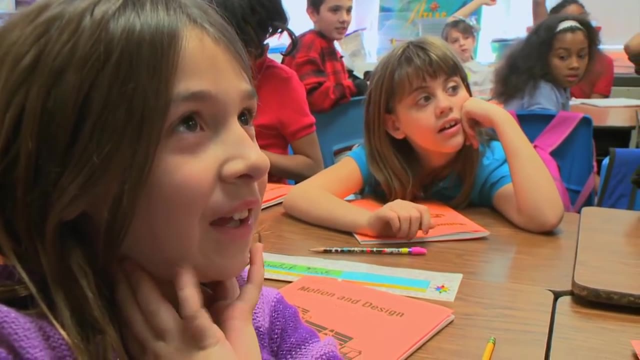 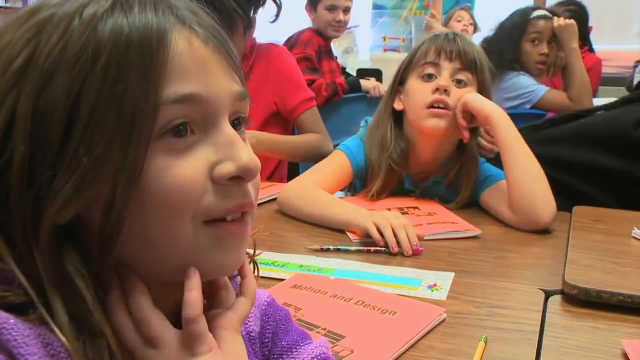 Okay, all right, You can kick it. Kick it, and what does that provide? A kick provides movement. It does provide movement. Is it a push or a pull? Push A push. What's your idea, Drake? Gravity. 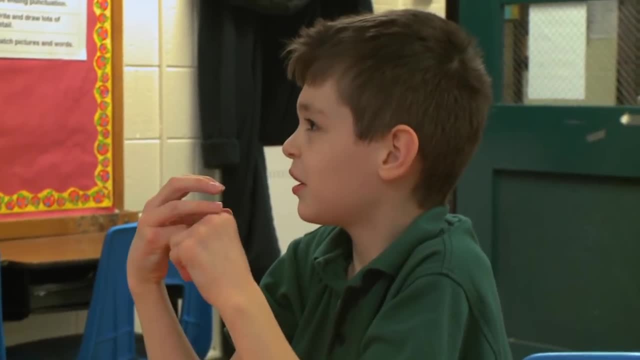 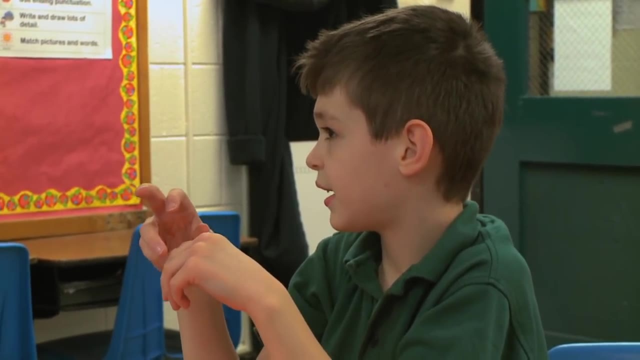 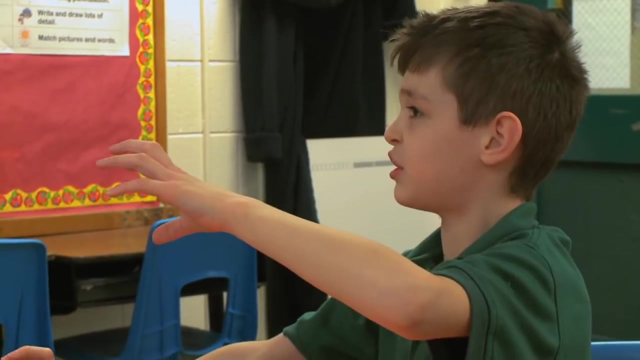 Gravity, and what kind of force does gravity provide? Sort of like a pushing, like a ramp or something could. maybe Does it push or does it pull. It kind of pushes it a little bit. It does a little bit of both, because at the beginning it pushes it down. 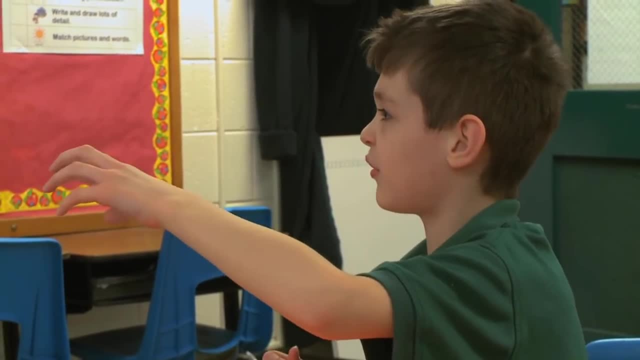 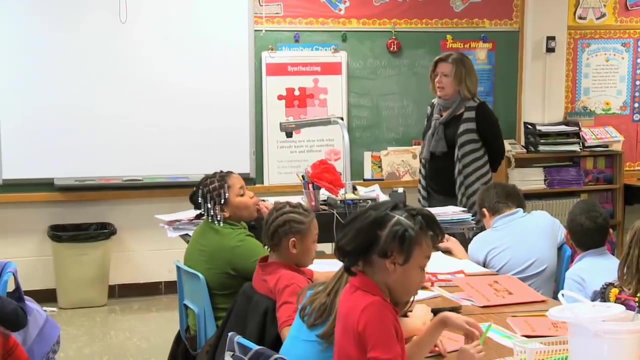 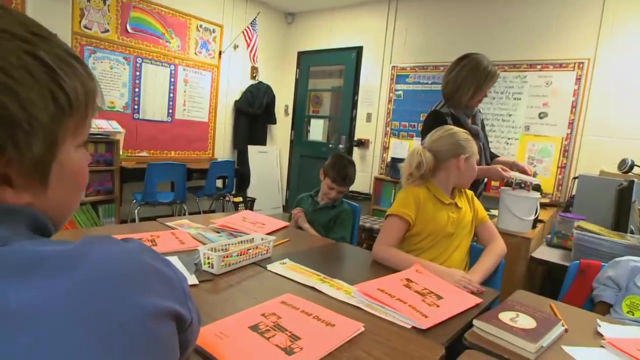 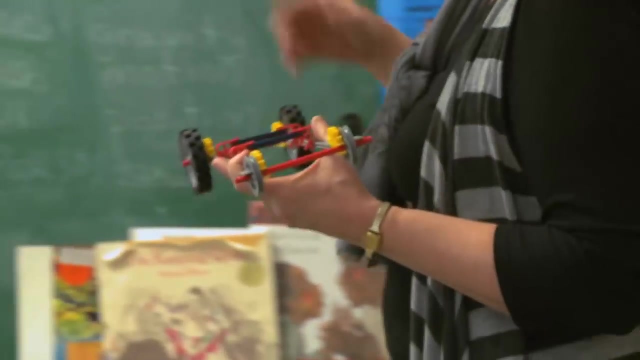 but then, after it pushes it closer to the end of the ramp, it'll start pulling it down. Okay, all right, Good, One thing I want us to think about: I'm going to use this vehicle here. Okay, Now we have done some reading and we have used some of our reading strategies. 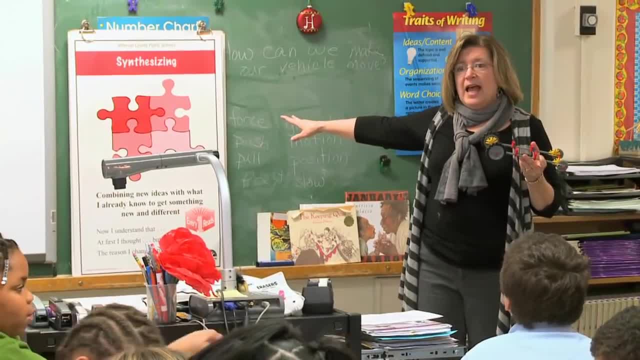 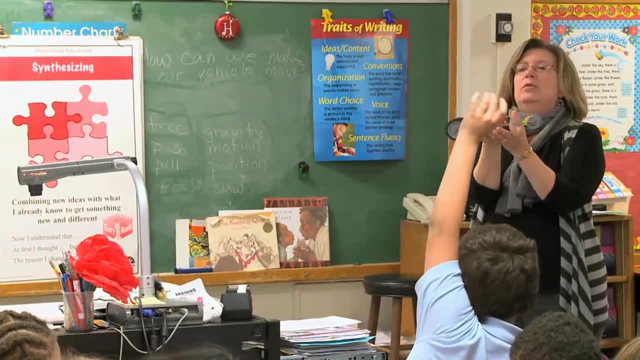 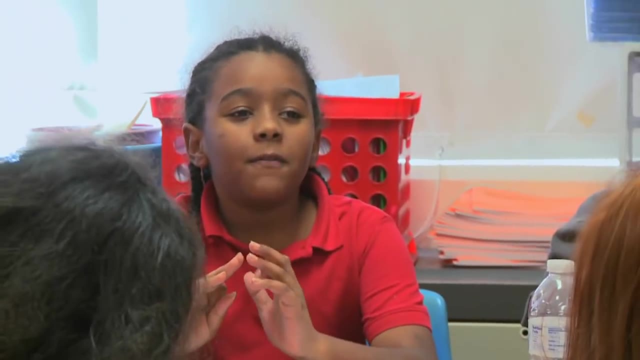 such as synthesizing. We got some new ideas and one of Tell me some things you found out from our reading that has to do with forces in this vehicle, Ramon Ramon. First I thought with the vehicle, with the vehicle we can use, like it's just like a toy car. 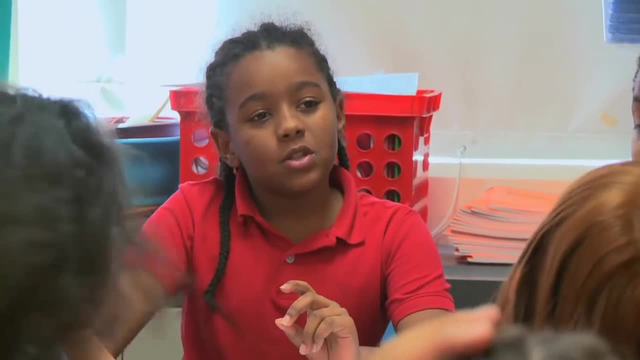 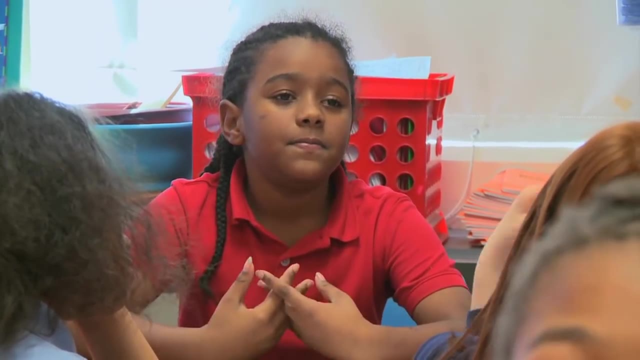 If you race in two toy cars, when you push them they keep going until they hit something. When they hit it, it stops. Okay. so a force provides the motion, It makes it go right, Okay, whether it's a push or a pull. 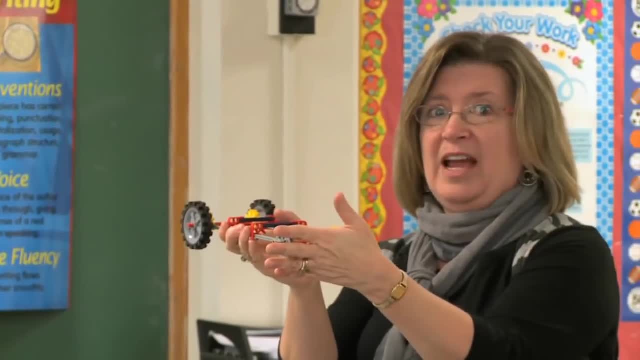 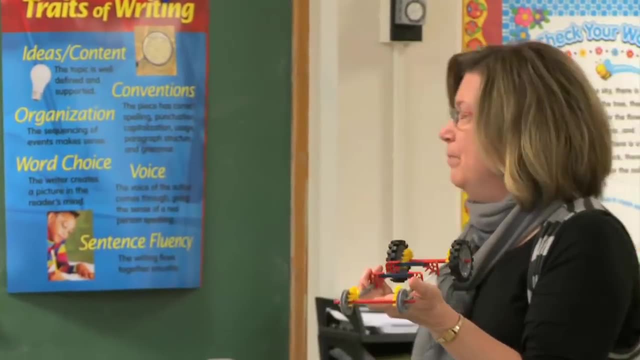 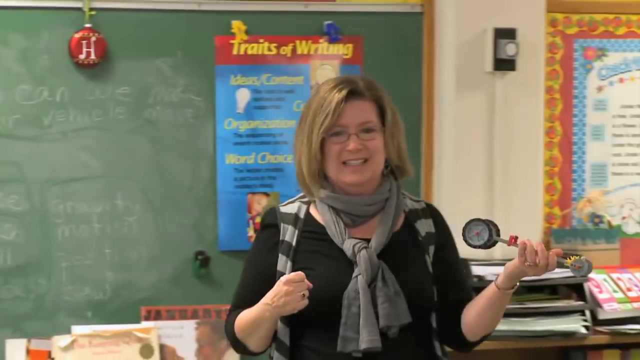 And then until another force, like you, said something. Has it stopped or changed? Good job, Good job. Stop or changes position- Okay, good. What else did we learn from our reading this morning? What other new ideas or things that you understand did you get from your reading? 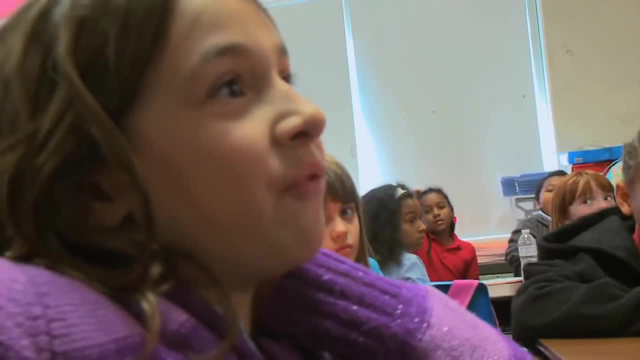 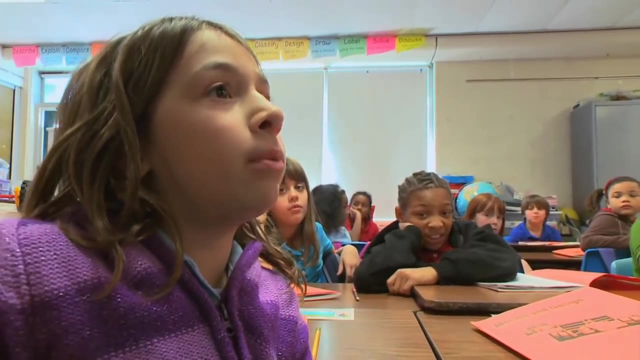 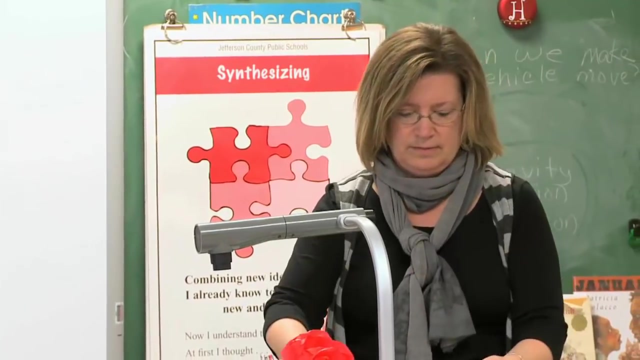 Isabel, I understood that because I thought, like a force was just anything, but all it was was a push and pull. Okay, Okay, Okay, Now I want you let's look at, let's look at this vehicle right here. 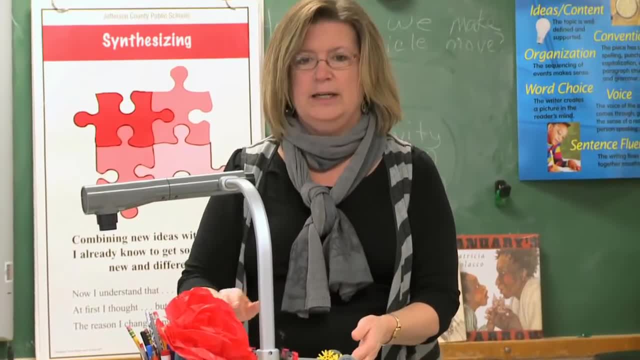 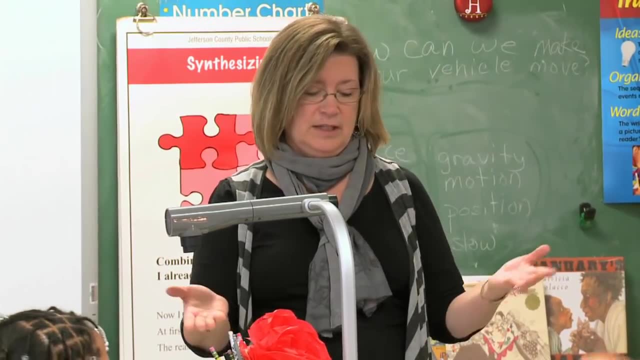 Okay, we've got everything on here. Let's look at this vehicle right here. It's not going anywhere. Are there forces acting on this vehicle? Because it's still, it's at rest, It's not moving. So is there force still here? 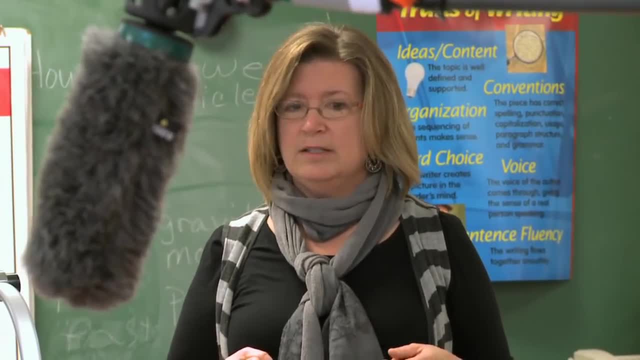 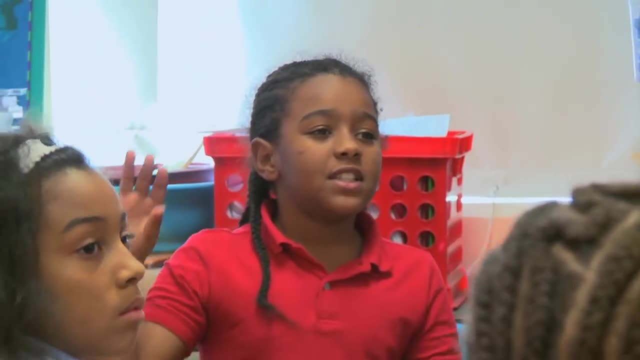 Yes, No, No, okay, Oh, somebody has a different idea? Yes, because It's force that's still moving it, but there's not enough force to push it or pull it. Okay, all right, There's still force. 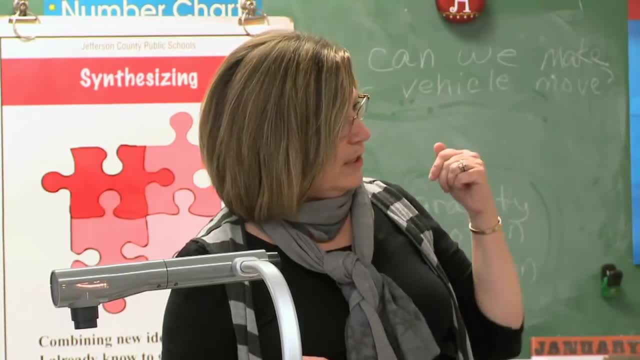 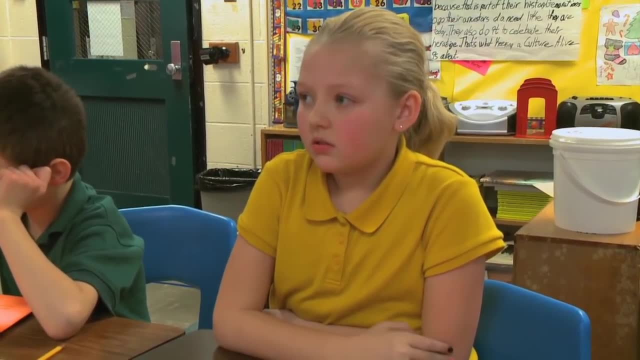 There's still force there. Okay, What's your idea? There's still force on it, but it's an equal amount of force. An equal amount of force. What does that mean? So the equal amount of force? what It's keeping it from moving. 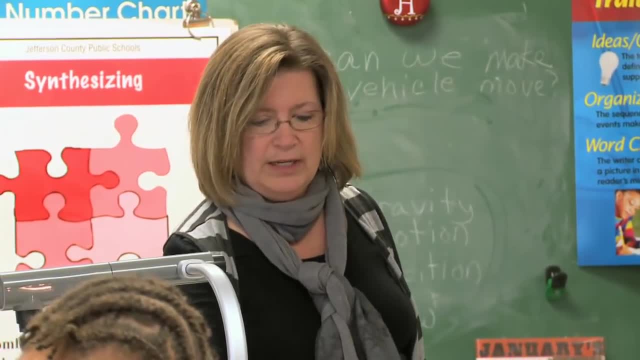 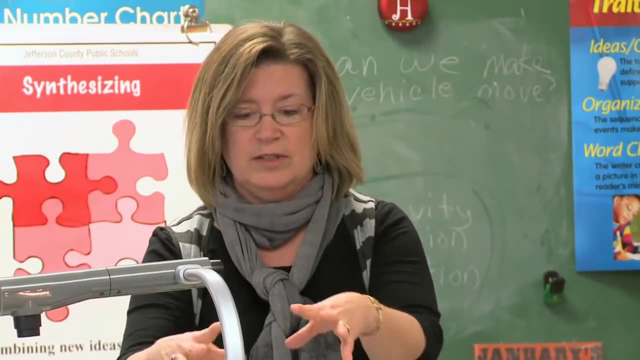 Okay, good, It's keeping it from moving. We've got gravity pulling on it, We've got this table in this book that's keeping it from going anywhere, And the force of the air. everything is equalized. Come here, Allie. 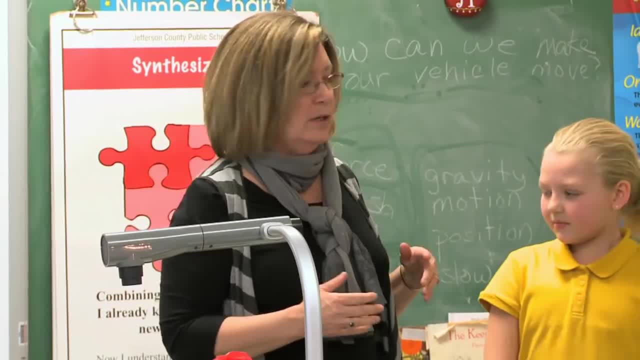 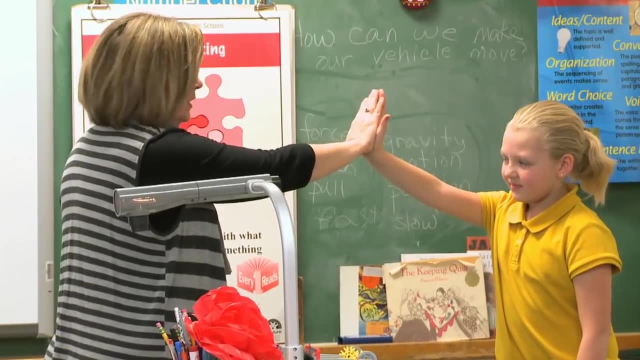 And when we have a balanced force, it's not going to move, It's going to be at rest. I want you to push as hard as you can. Okay, Are we moving? No, Well, I just moved my hand, but I mean, am I moving her hand? 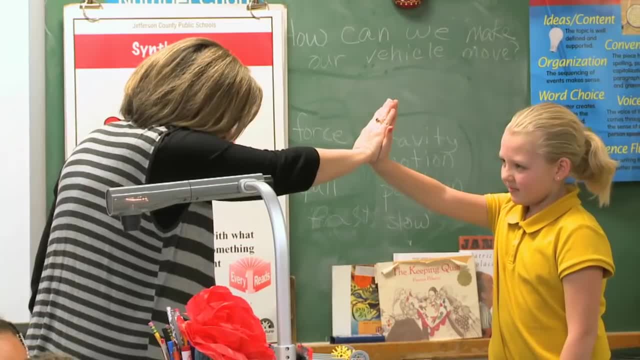 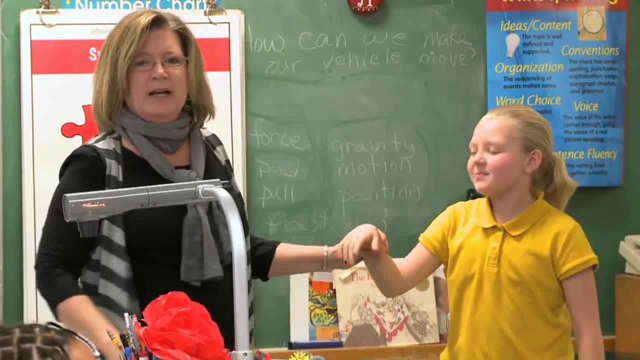 Is she. Are you moving mine? No, because we're going to push. Okay, Now we have equal balance of force. She can't move my arm back and I can't move her arm back, because the forces are equal. 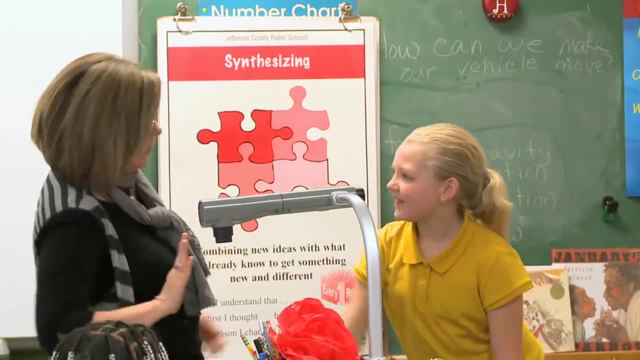 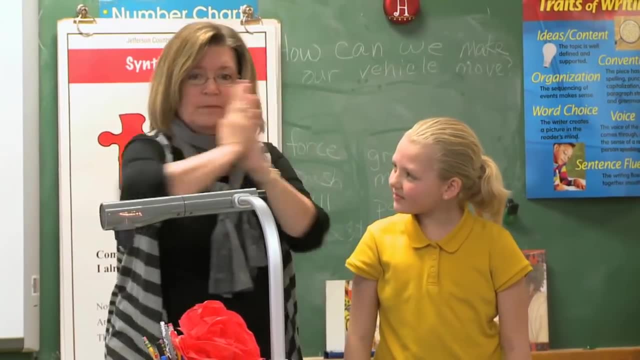 Okay, Now, push as hard as you can, Okay, Okay, Now, the balance was unequal. She had more force on my arm. That unequal force forced my arm to move, which is what you were doing to the vehicles when you made them move. 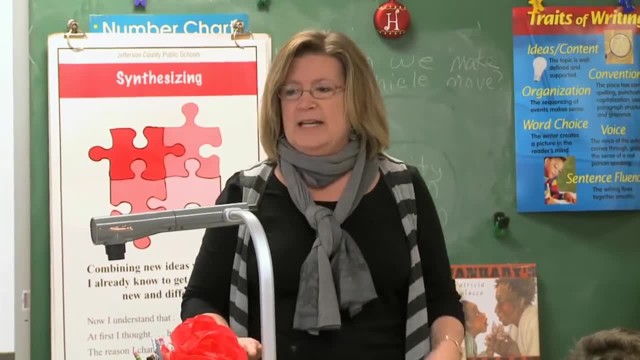 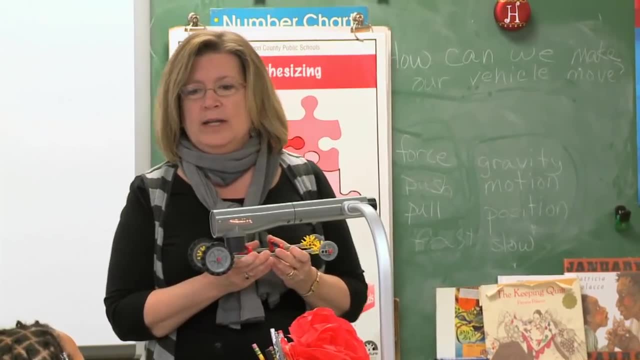 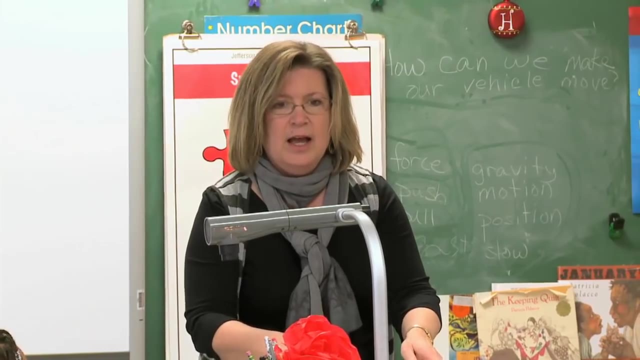 Thank you, sweetheart. What we're going to do today is we're going to test force on our vehicles. We're going to use what's called a falling weight system to do that. Okay, A falling weight system. Now I want all eyes to follow me over here. 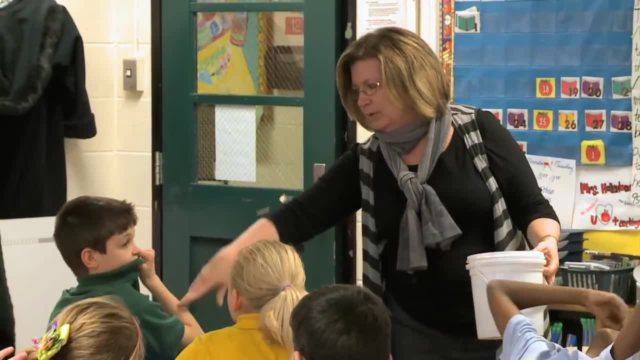 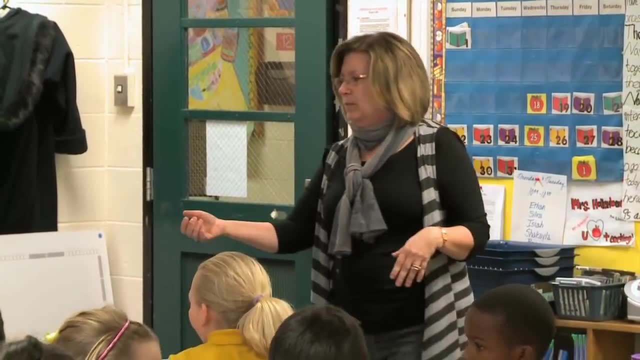 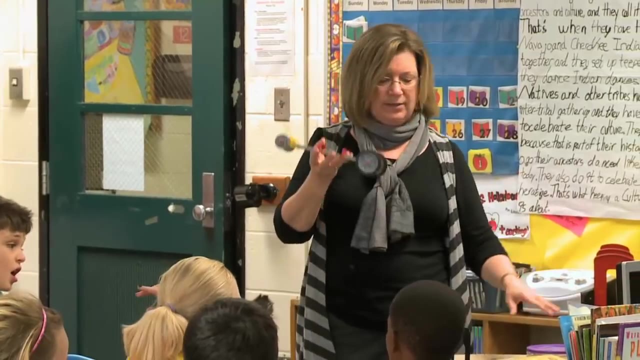 Okay, Okay, You will have. Would you get me my vehicle please, Or whoever's vehicle? Okay, You see, around the room we have. Thank you, sweetheart. We have placed our buckets and vehicles and some other equipment around the room. 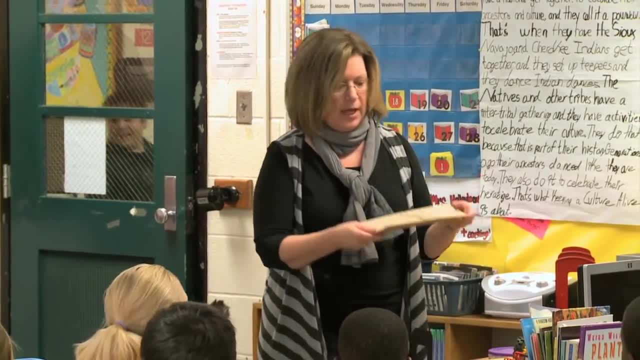 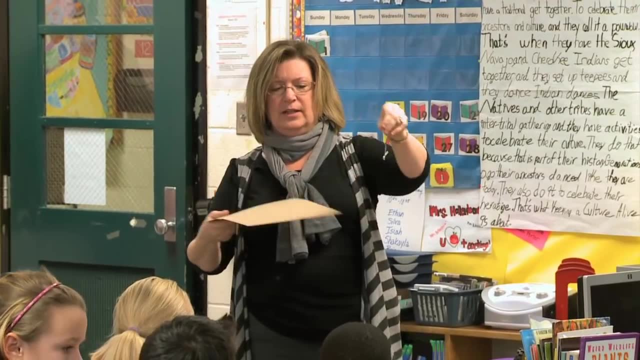 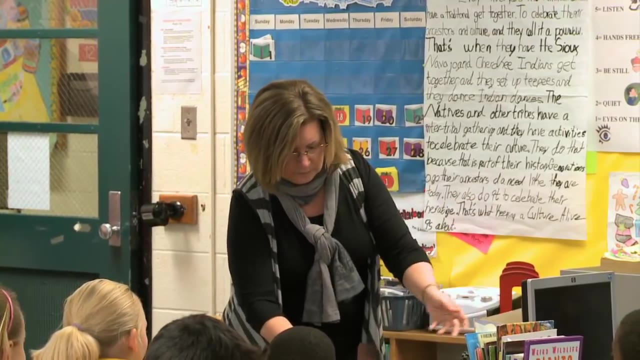 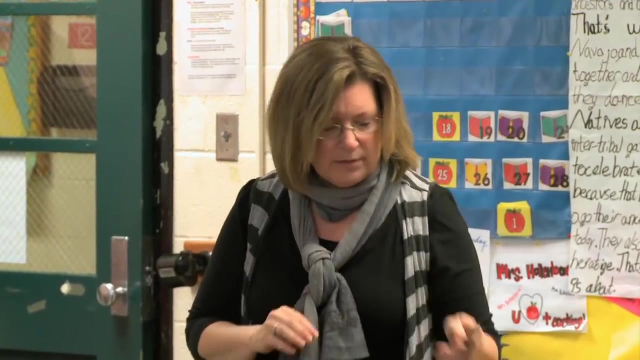 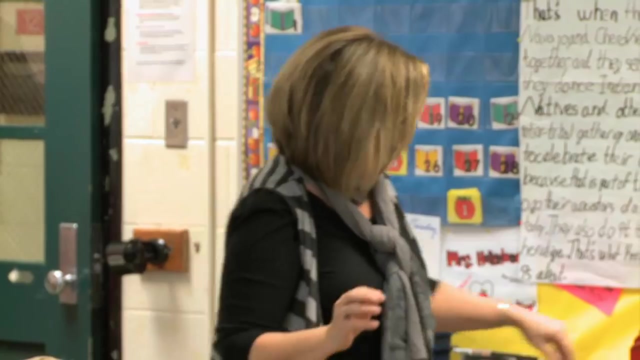 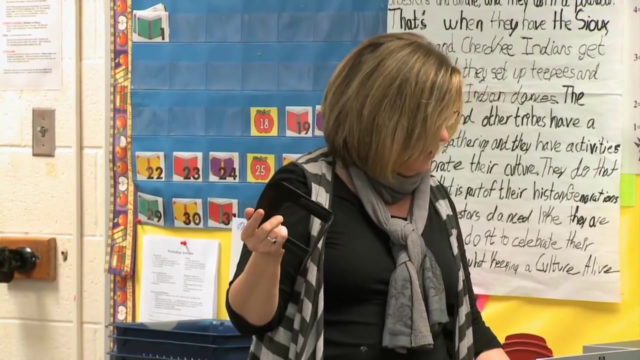 What I have is a piece of cardboard and it has some fishing line and hooks. Okay, You also have. You also have weights. Okay, And we have a bookend. Okay, And we're going to. Why would we have a bookend if we're trying to make our vehicle move? 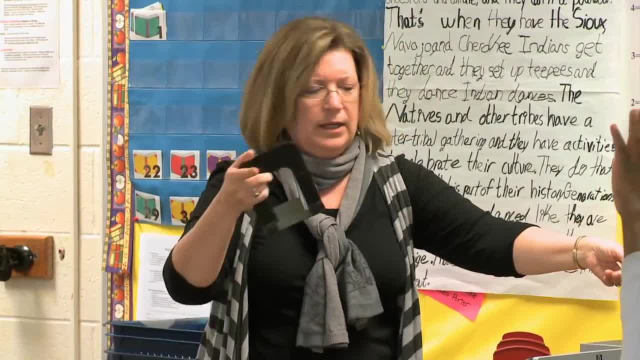 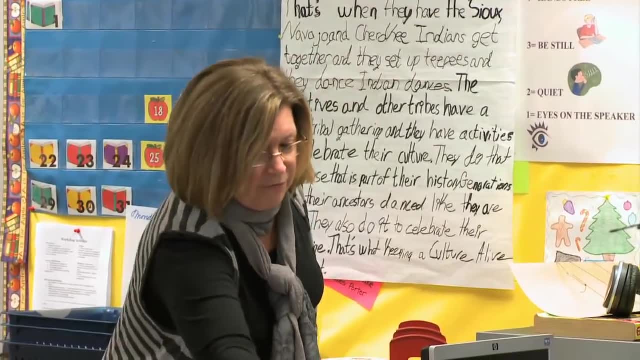 What's the bookend? What's the bookend for What? do you think, Ethan? To stop it? To stop, Stop what? The vehicle? Yeah, Okay, So it doesn't fall off the edge of our desk, of our table, of our bookcase. 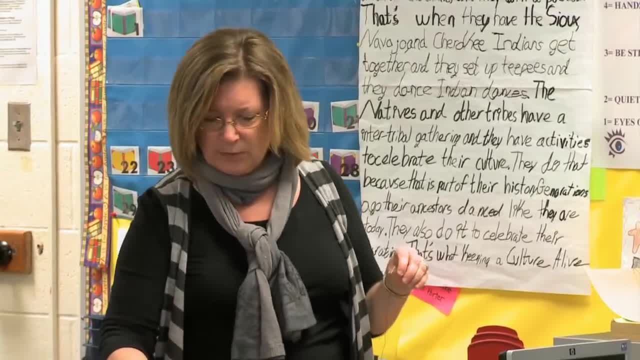 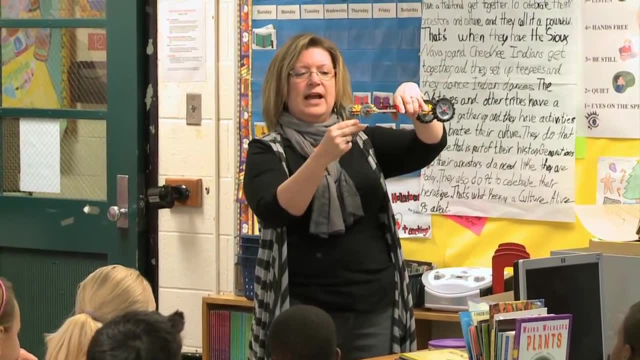 Now I also want you to think about as we're doing this. you're going to take the hook and you're going to put it against the front axle. Remember that front axle is not moving. You're going to hook it here. 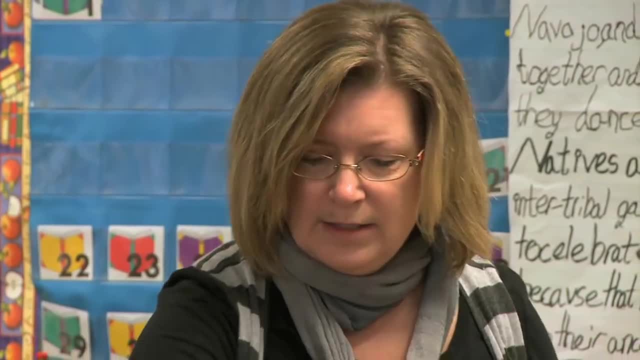 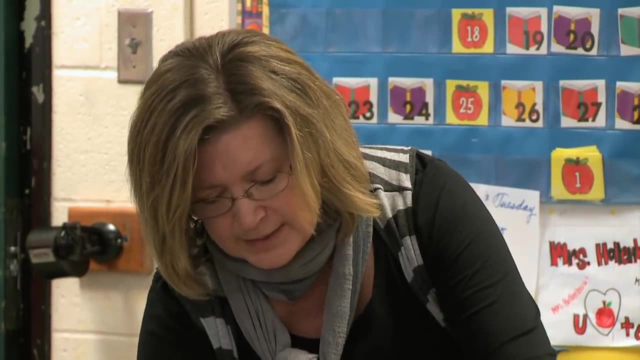 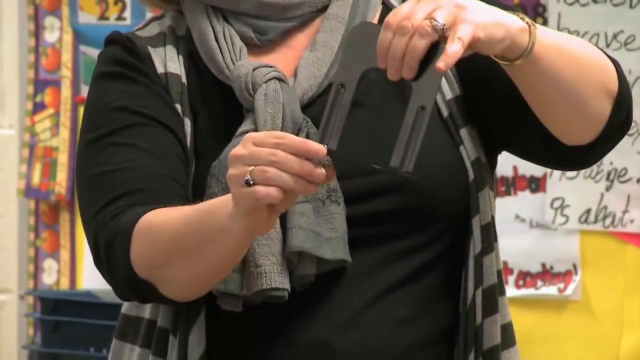 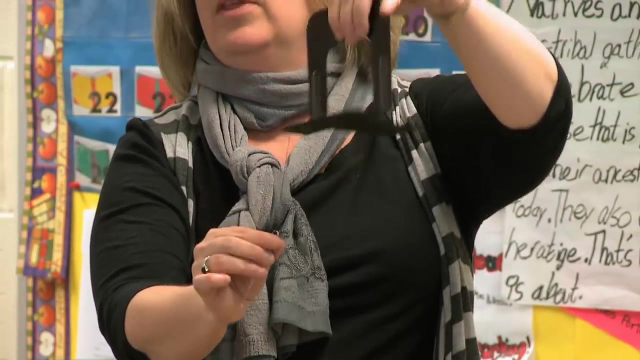 And you will have the other end right at the edge. Okay, What that means. I'm going to hold this up. Sit down, I'm going to hold this up. This should hang like this, where the top of this paper clip is just as equal, flush with the bookend. 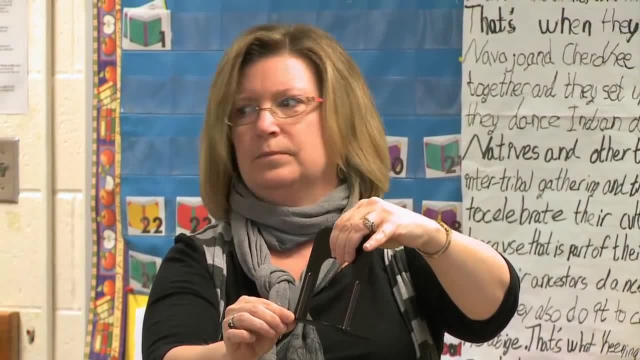 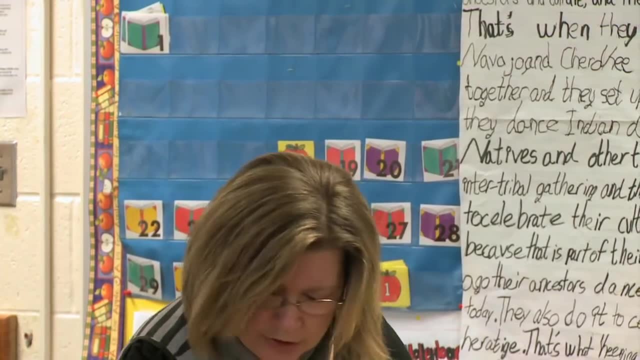 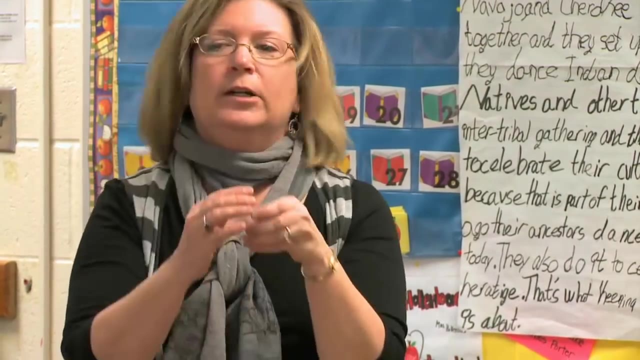 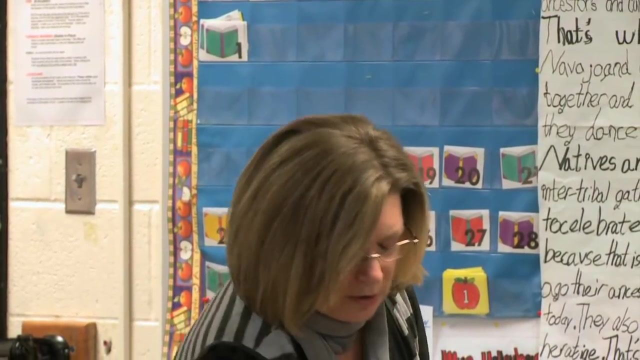 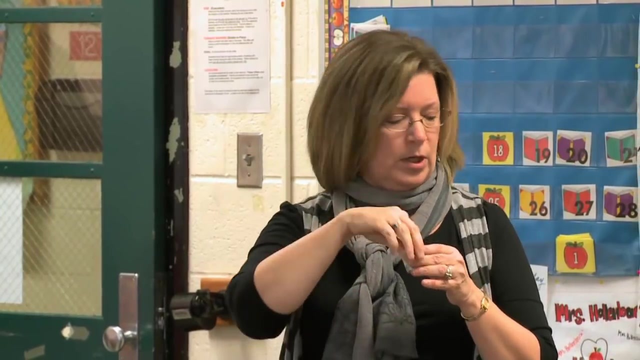 Okay, All right. All right, Put your, Put your hand down, please. Now you're going to be putting weights. You have little washers- 25 little washers in a cup- and you have one large washer. In a few minutes we're going to be reading our instructions as a team, but I just kind of wanted to show you how this worked. 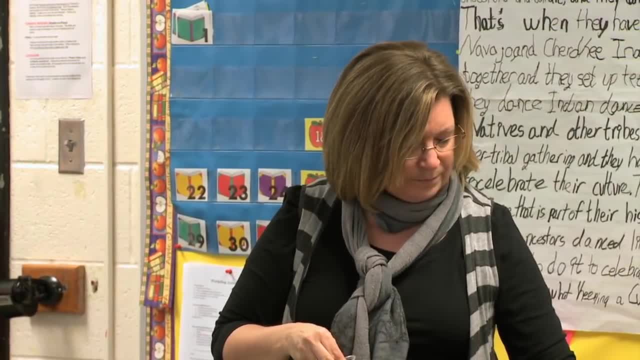 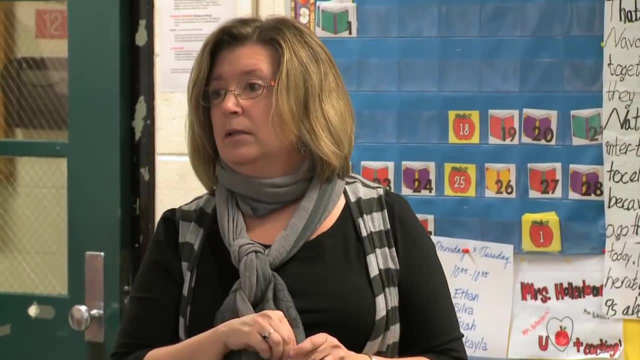 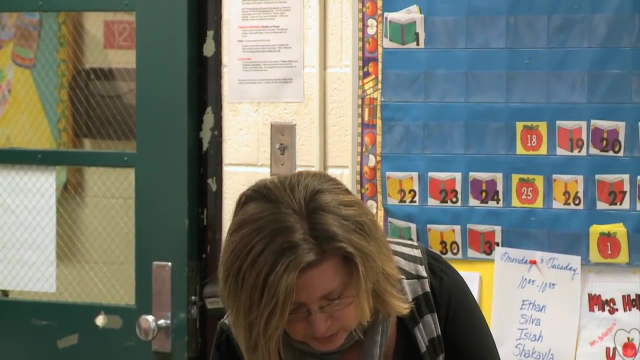 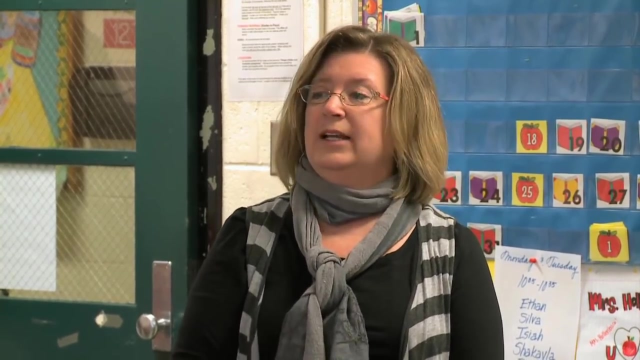 Someone's going to be holding our vehicle while another one is putting on a certain number of washers. Okay, Someone will be holding this, holding the vehicle, You're going to place the washers on the hook, and then one of you is going to say: 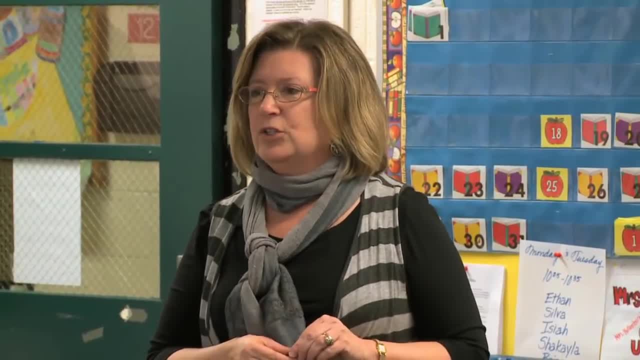 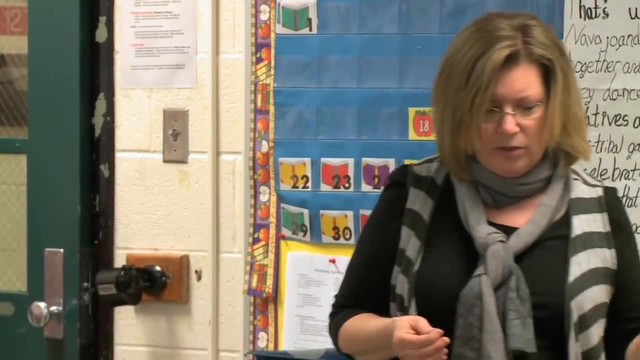 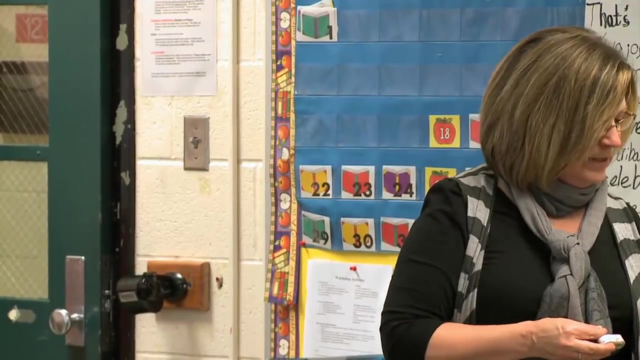 Go, You're going to let go and you're going to see how far it travels. Okay, You're going. well, how do we know how far it travels? I had- You will have also a tape measure, Okay, In which you can travel a distance. 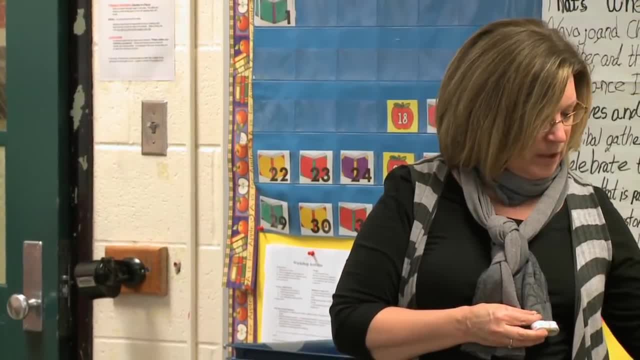 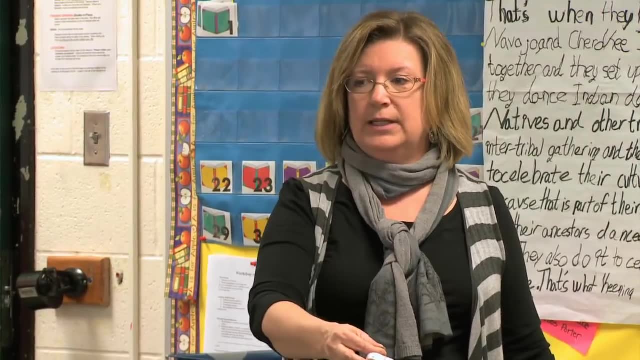 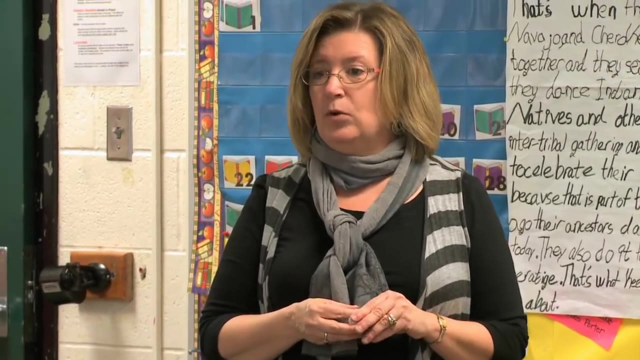 You can use. Make sure that you mark where the back tires are so that you know how far it goes. Put hands down, please, So that you know how far it goes. Put hands down, please. And then you're going to record in your journals and I'll show you how to do this. 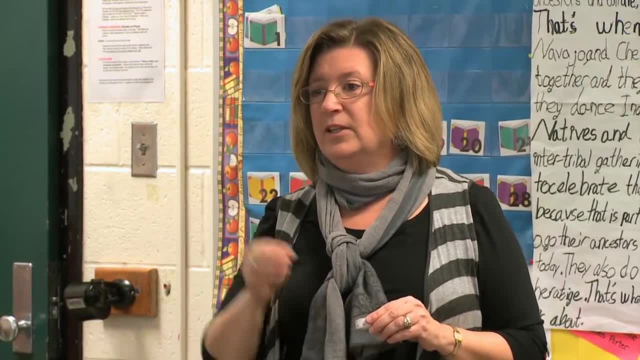 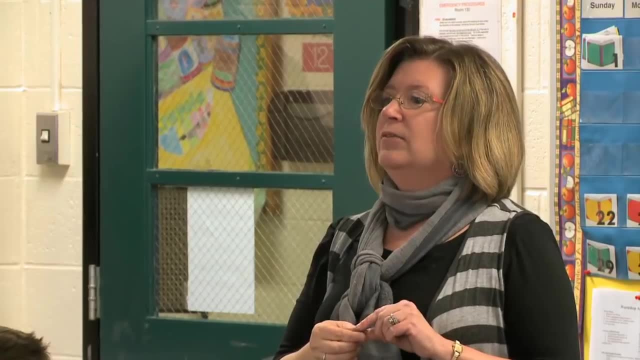 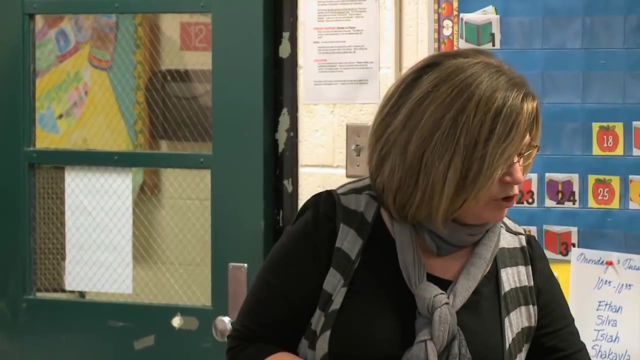 You're going to record in your journals what you found. Then you're going to keep increasing the weights. I want you to think about it. If I have four small washers Silva and I put it on the hook, how is the effect of the motion on this vehicle going to be different than if I had eight small washers? 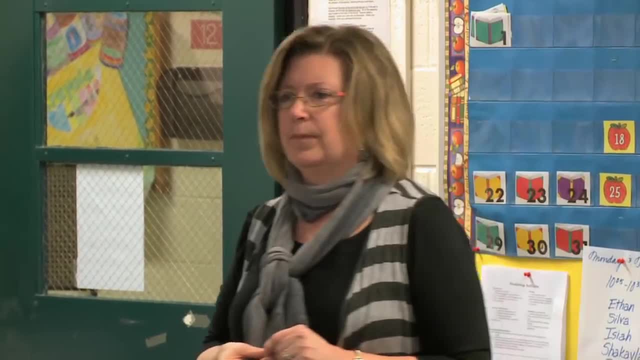 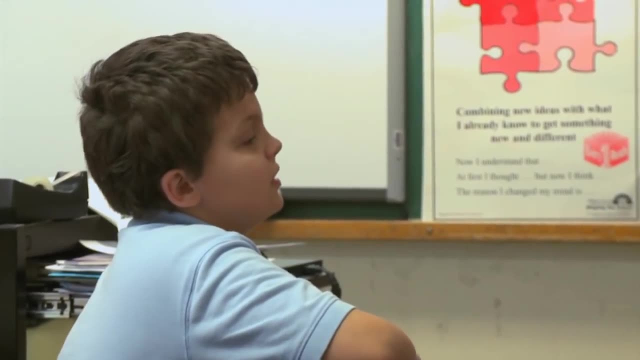 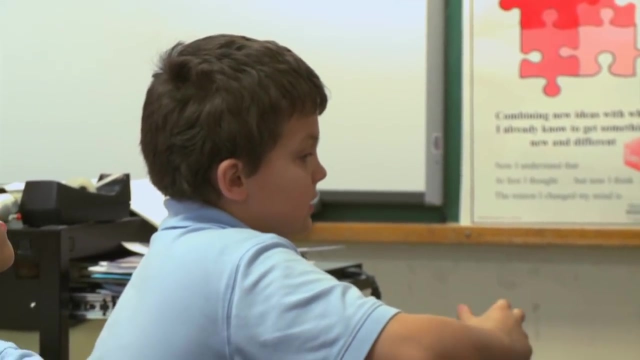 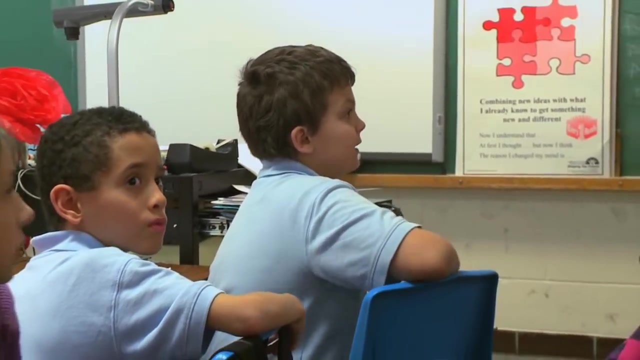 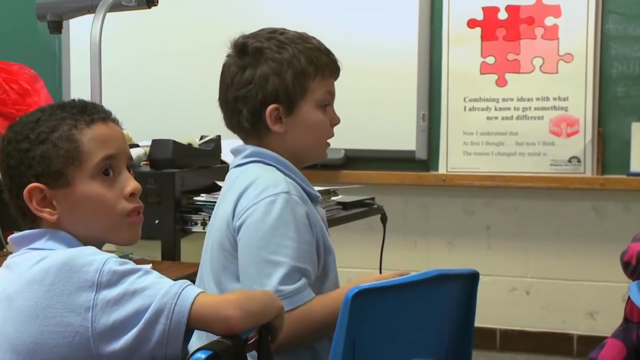 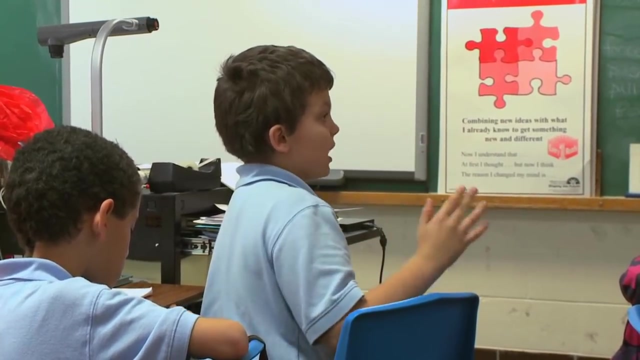 How is that going to be different, do you think? Or would it be different? Yes, It would be different because the weight is kind of like helping the gravity stop being the vehicle and pulling it down. So if it has four weights It'll go farther, but if it has more weights it will stop sooner. 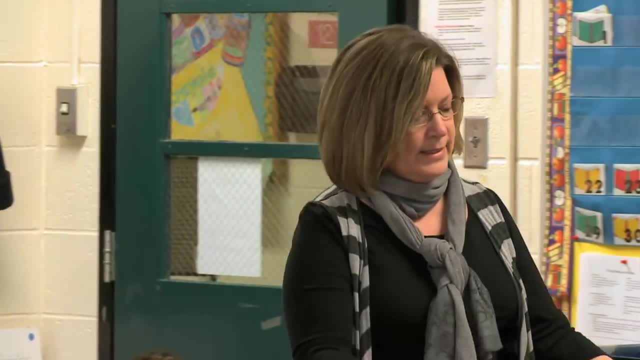 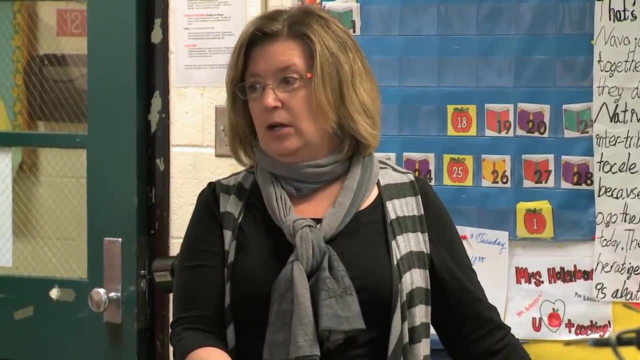 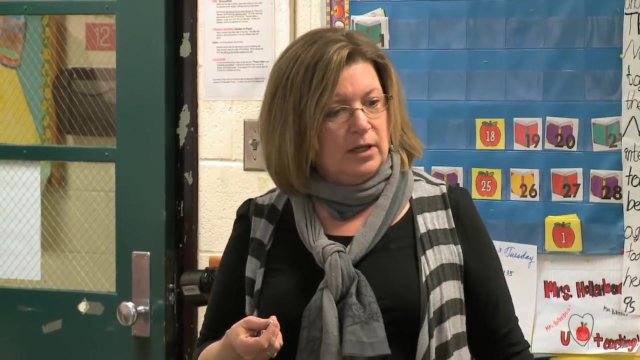 Okay. Okay, so you think, the more weight it'll stop sooner. so it doesn't go as far. So the less weight, the further it goes. Who has another idea? Okay, I like your thinking. Yes, The more weight it puts on. 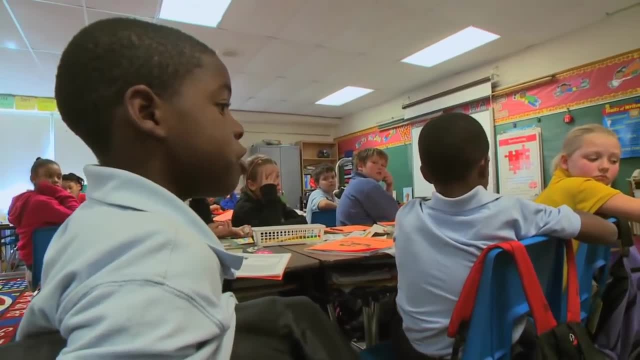 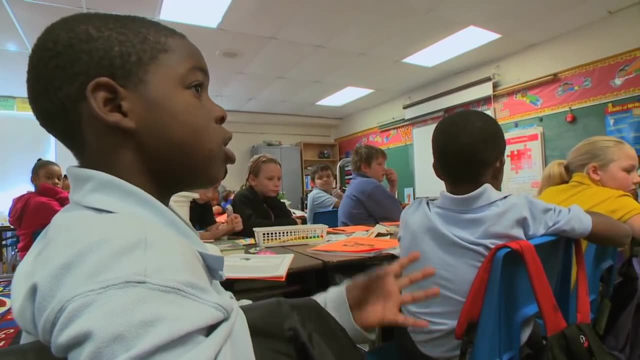 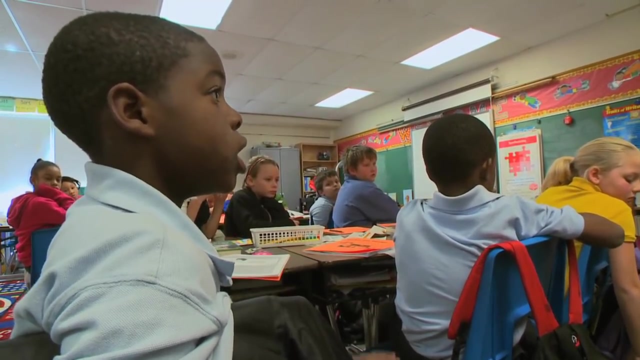 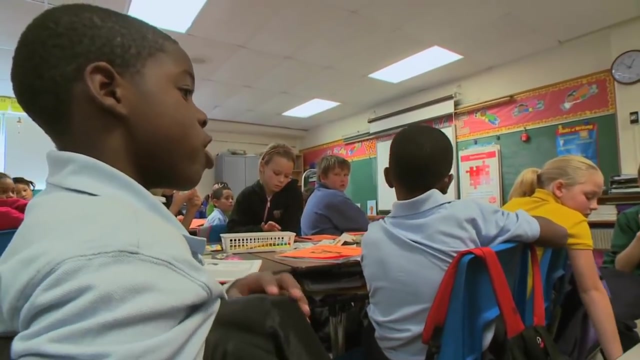 The faster it's going to hit something, because once you put the washers on there, the hook's going to start moving down, and that's a part of gravity. Very good, It's going to start moving down, then our car is going to start coming. 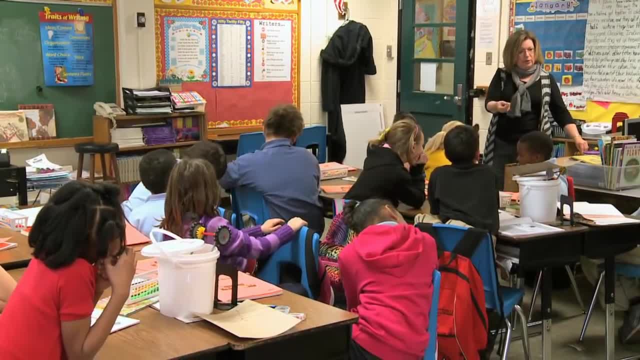 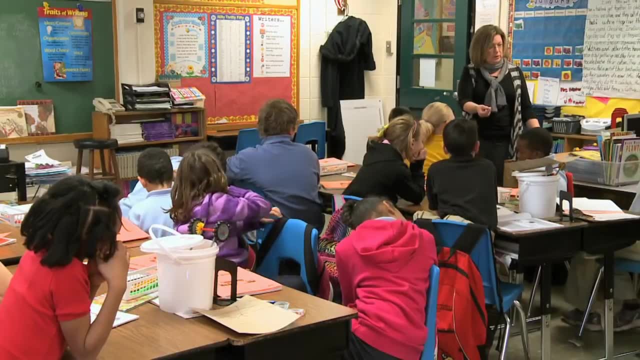 Okay. So what's going to happen? The more weight I put on there, how's that going to change the motion of the vehicle? The more weight, the more what? The more faster it goes, The more speed, the faster you think it'll go. 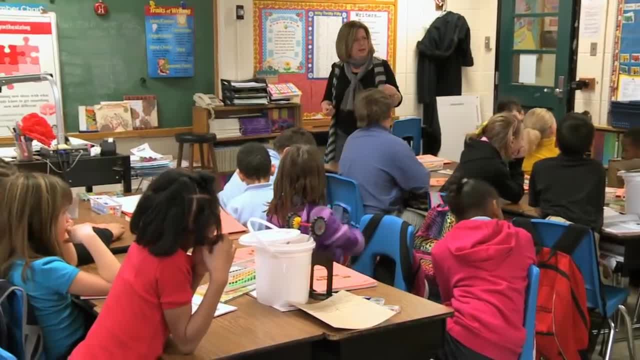 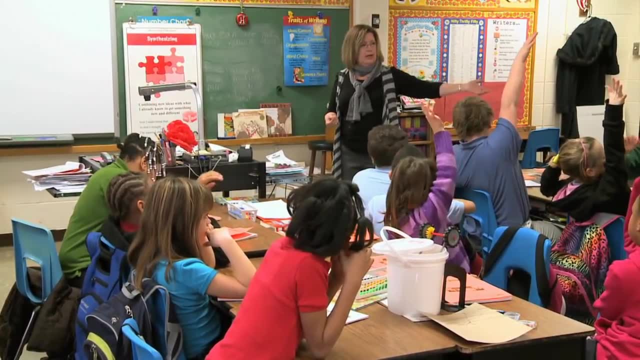 Okay, Well, we can see about who agrees with Jackson that the more weight, the faster and further the vehicle will go. Okay, So we have. what about two, three, four, five, six, seven, about ten, Ten? 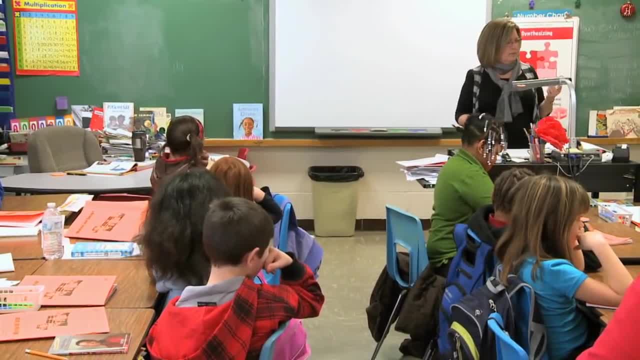 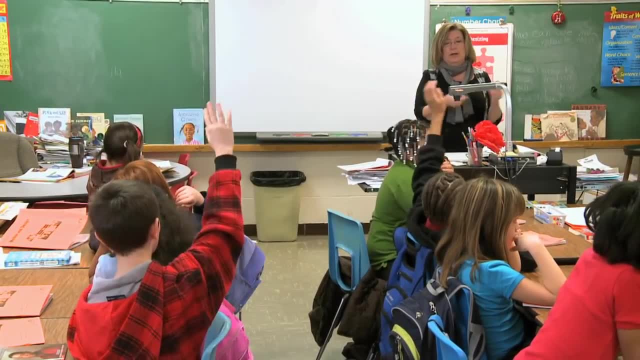 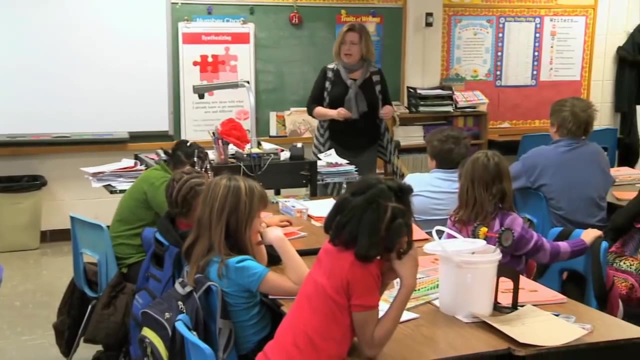 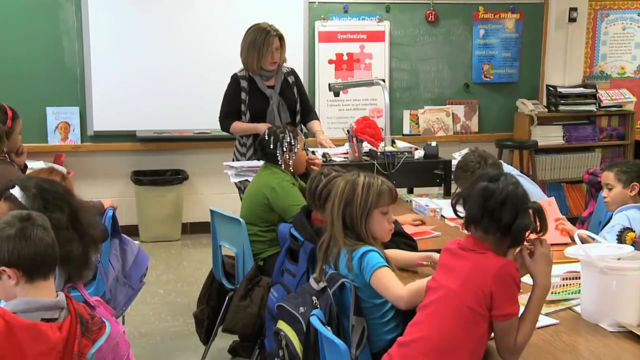 Who agrees with Jaden that the more weight the less, it won't go as far. Okay, So we're going to see, We're going to find out. I would like you to open up your journals to page 13.. At the bottom it says page 13.. 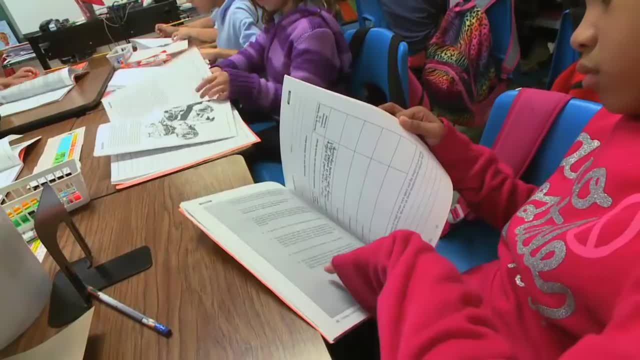 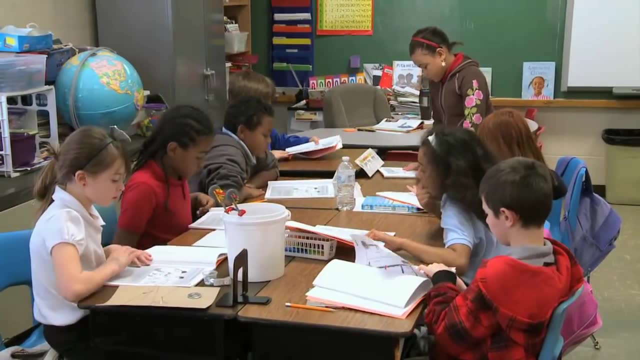 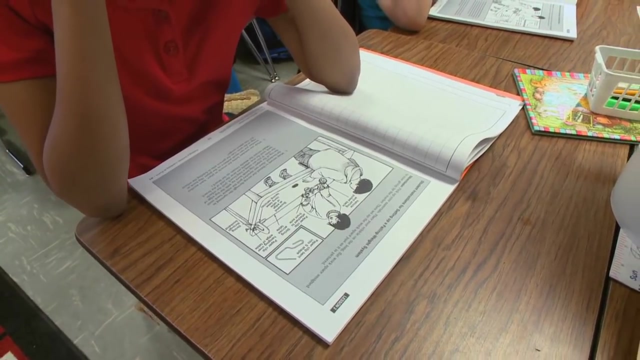 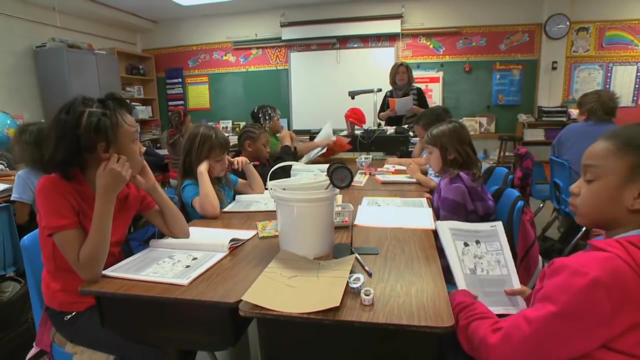 Open your journals to page 13.. Okay, If you look on page 13.. Oh, my camera's not working If you look on page 13,. who would like to read the first part of the directions? Because the first part we've already. 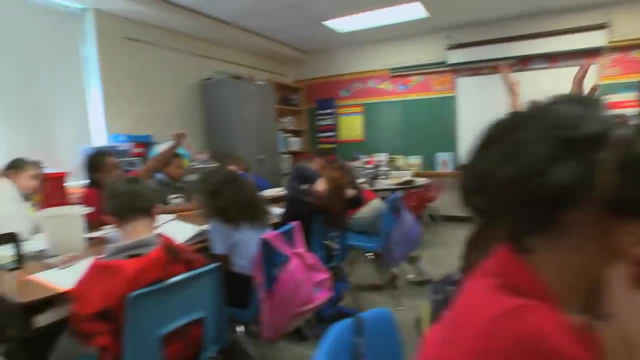 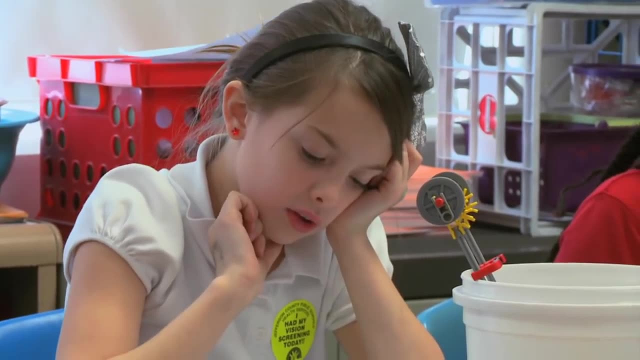 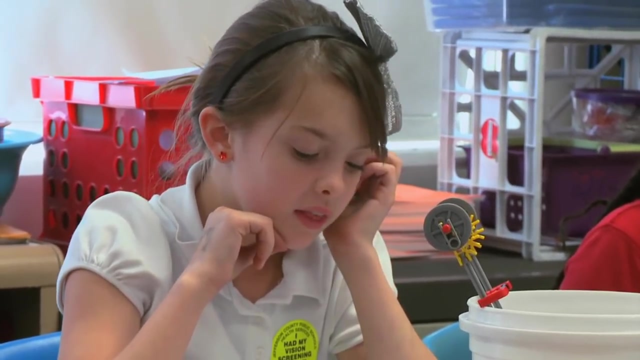 We've already kind of have for us. Read the first part of the directions Keely. Pick up the materials, Place your vehicle on the long flat workspace assigned to your group by the teacher, Then set up the workspace just as it is pictured. 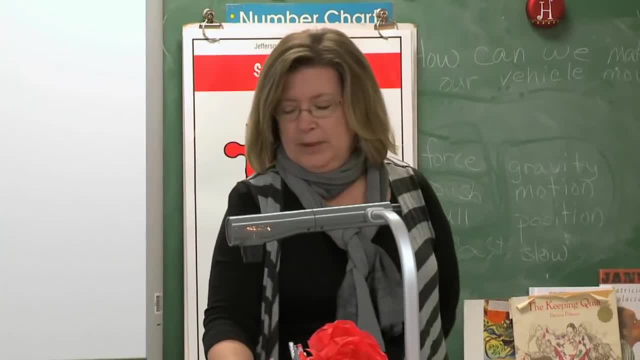 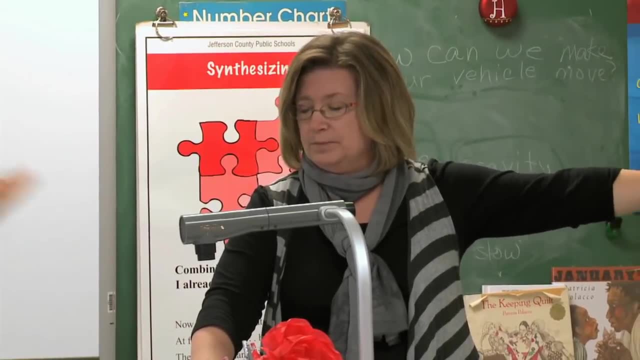 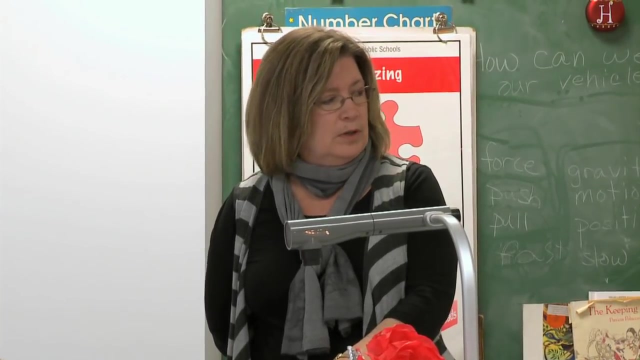 Okay, Now, if you notice the picture, what did you? the picture kind of looks like what I showed you, isn't it, Didn't it? Okay, The picture was just like I showed you. Now you're going to. you're going to read, in your group, the steps. 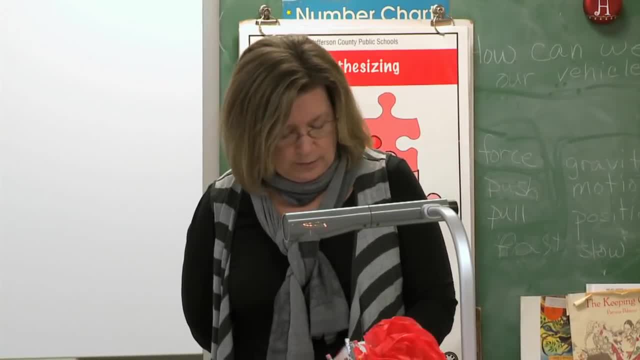 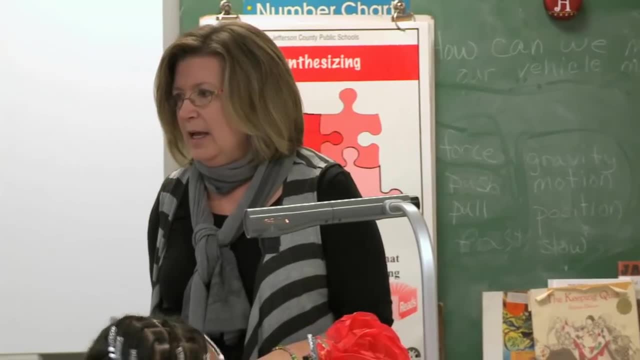 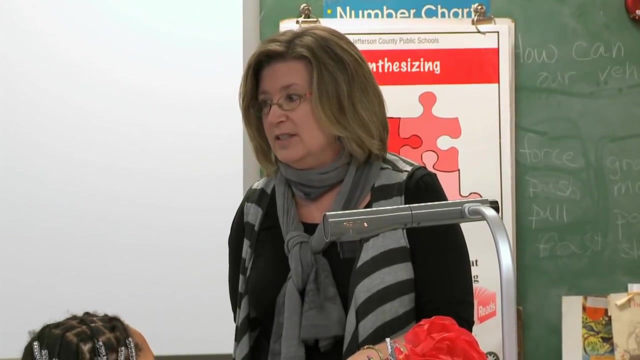 Okay, One, through pages 13 and 14.. And I want you to talk about. you're going to read it through And then I'm going to assign you to your spots And you're going to follow these directions. You're going to follow these directions to complete the assignment. 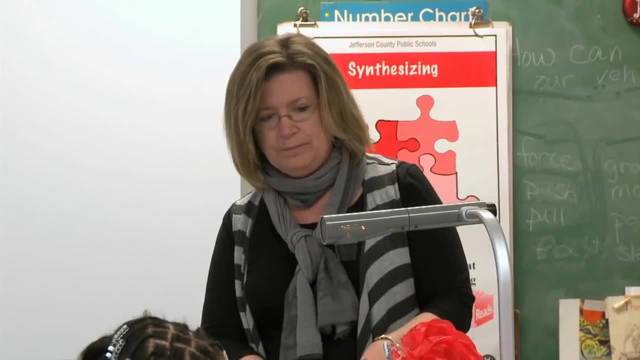 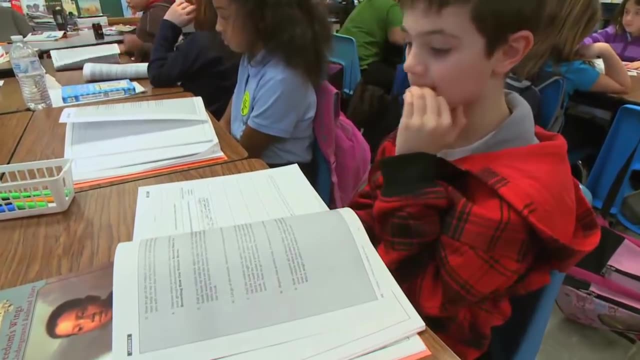 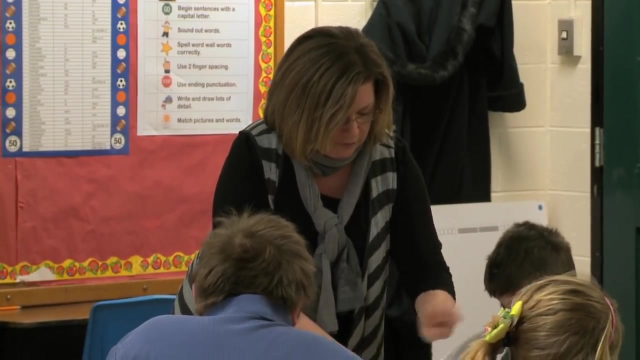 Now I want you to look on page 15 in your journal. Look on page 15 in your journal. Okay, This is your recording sheet. Page 15 in your journal is your recording sheet And I want you to look carefully at this recording sheet. 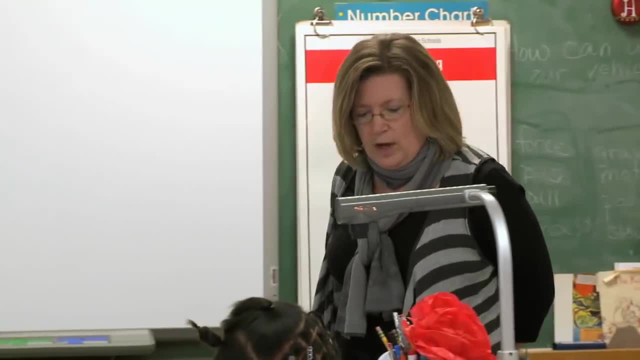 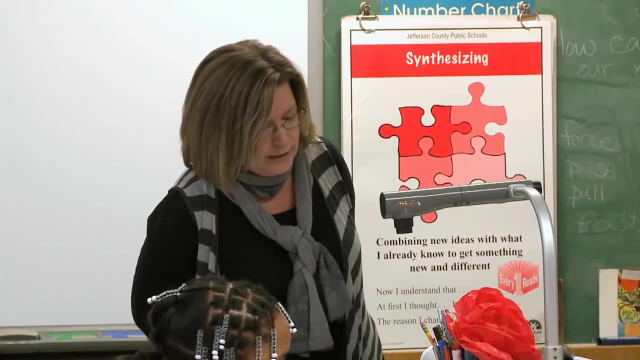 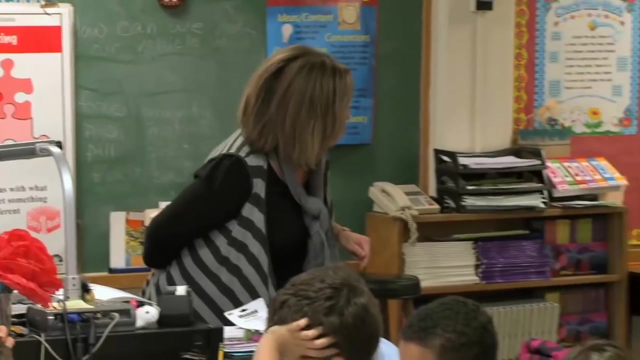 Now, if you notice the recording sheet, what is it? We're recording how our vehicle moves And we have three columns. One column it says number and size of washers. So it's giving you how many washers you're going to use and what size you're going to use. 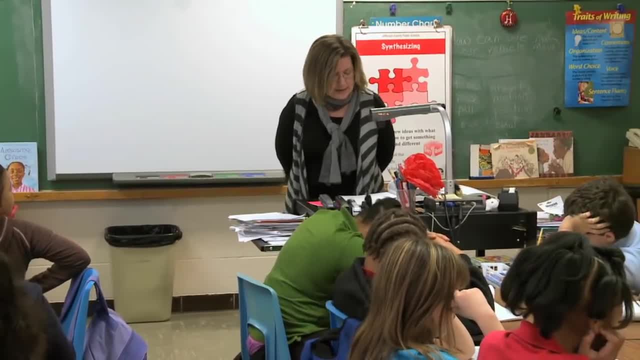 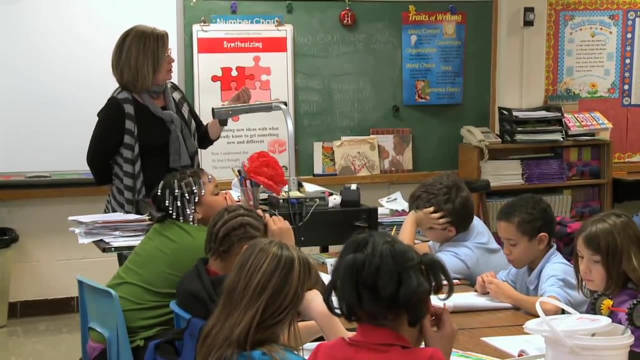 Okay, In the middle you have a larger space. That's observations about how the vehicle moved. You're going to write down what you see. You're going to talk about it. Write it down, And each one of you will be writing it down. 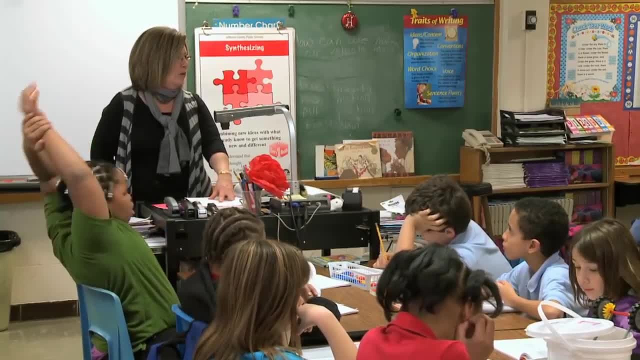 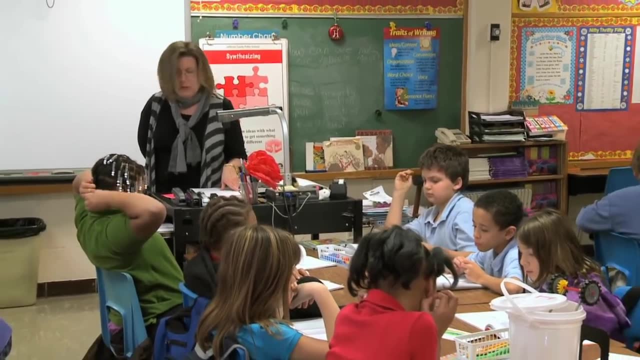 And one person from your group will be sharing out once we're finished. Okay, Now I want you to look at this first one with one small washer, Because you don't have to use one small washer. This is already showing it to you. 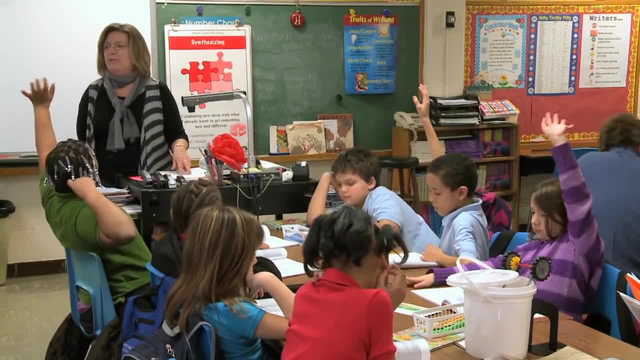 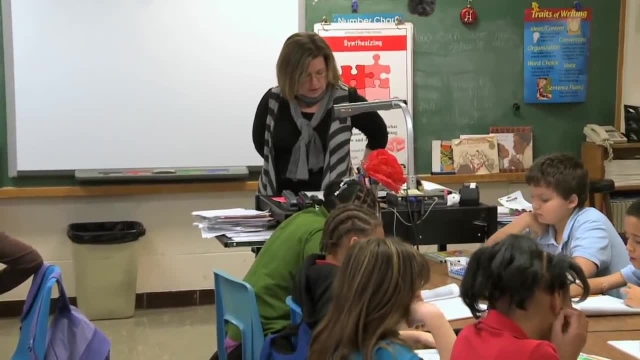 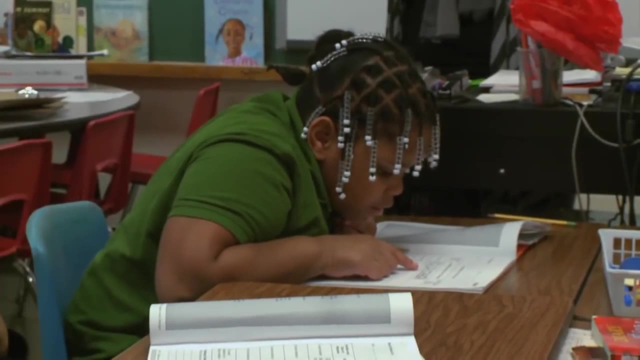 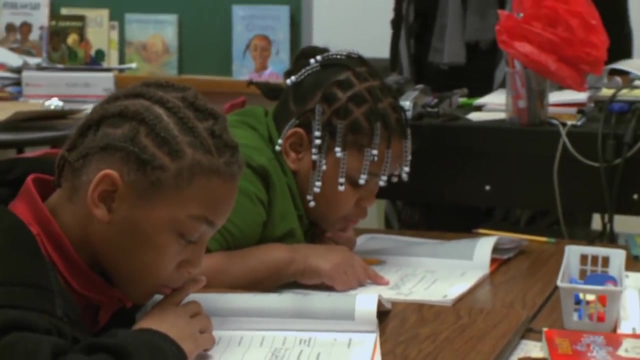 It says. who would like to read what the fourth grade observer wrote in that area? There was only a small For pulling the car. First it wouldn't Start Start moving, Then it moves very slow. Okay, So that's one thing. 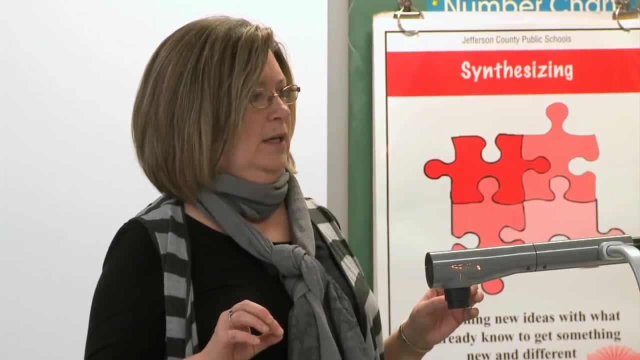 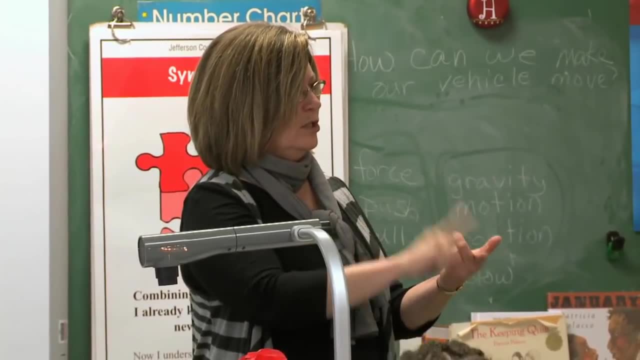 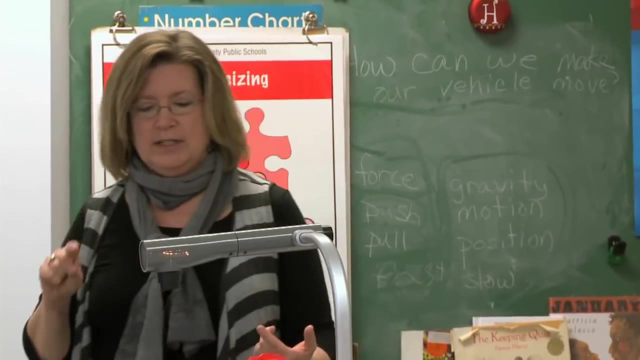 If you find that it's not moving, okay, don't give it a push. But you can one finger touch the back axle and see if that helps, Okay, Okay, Okay, Just give it a touch, Don't push it. 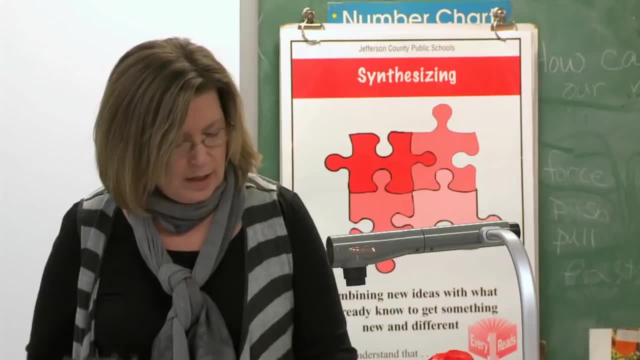 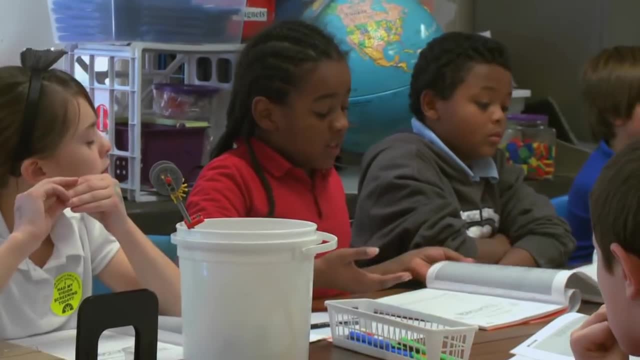 Because you wouldn't get a true reading. Okay, So you're going to? Yes, I have a question. Yes, As you set it up like you set it up just like it, but I don't know how do you? 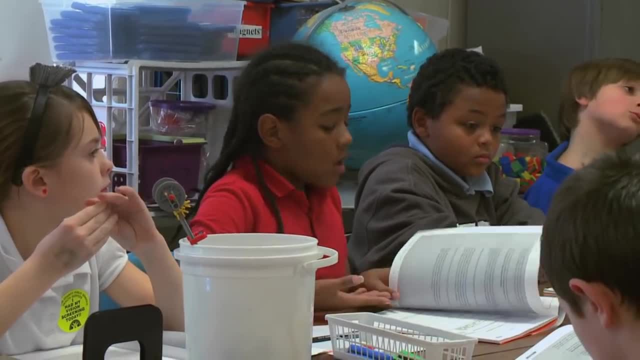 When you pull it back. how do you do it? What do you mean when you pull it Like, how do you possibly let it go? You pull it up, You just let it. You put the washers on, You let it go and see if that'll. 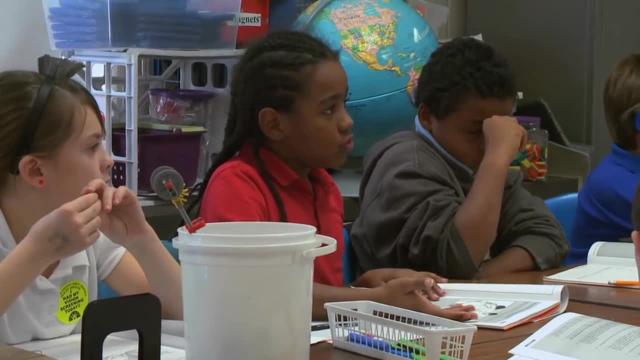 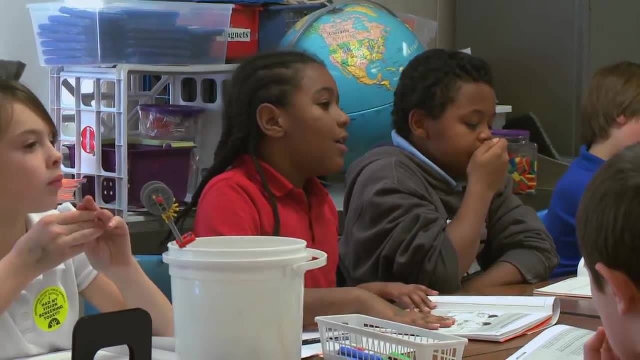 You let it go and see if that'll pull the vehicle, and see how far and how fast it'll go. We're going to see what it does to the motion. So you pull it backwards If it changes. No, The string. 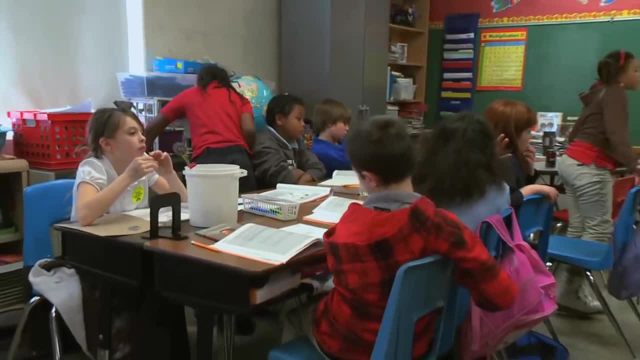 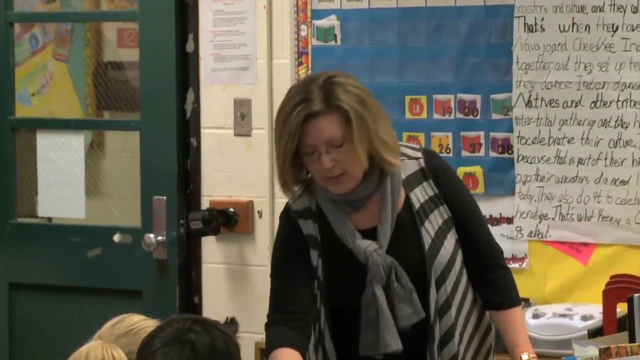 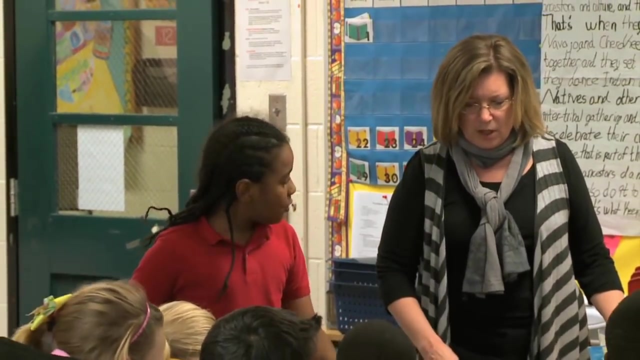 Come here, Ramon. The string is pulled tight. Okay, Now I don't have anything on here, so there's nothing pulling really. this. Okay The vehicle. Okay, Let it go backwards, So no, Someone's holding it. 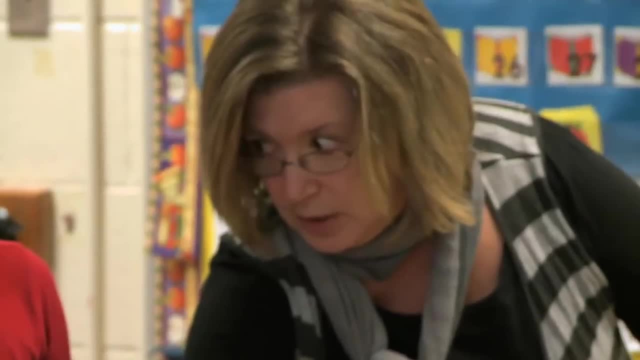 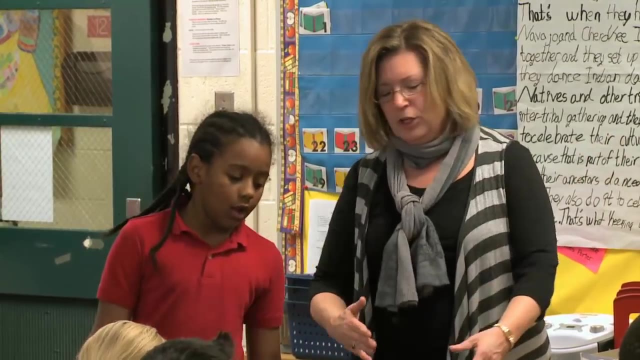 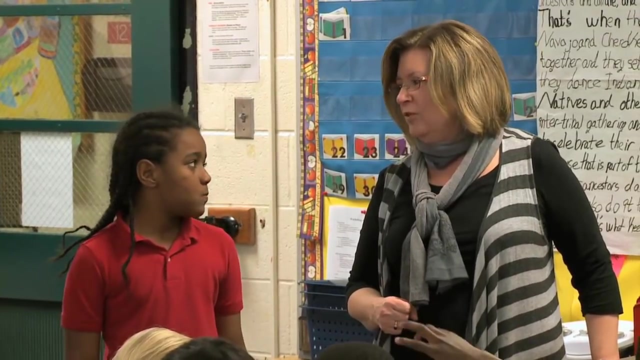 Once you put however many washers you're going to put on here, whatever it says, then you're going to let it go And then you're going to see how far and how fast it will go with however many washers you put on there, whether it's 4,, 8,, 16, or 20.. 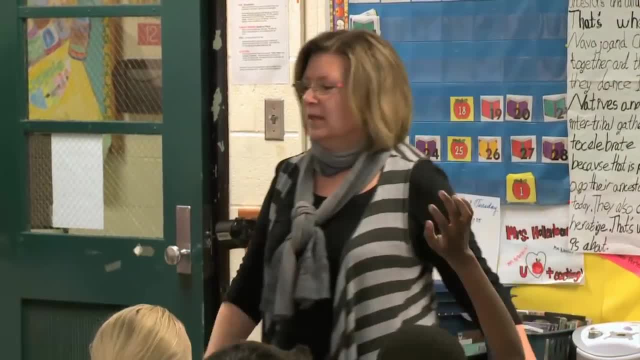 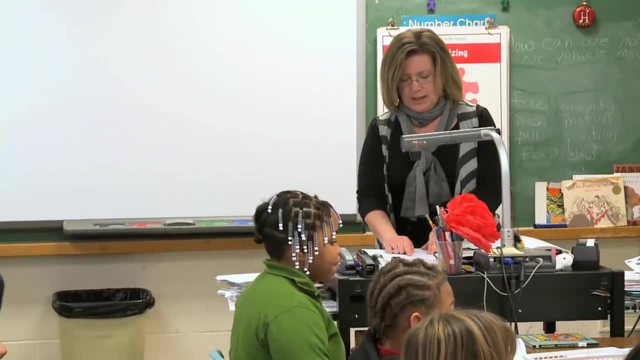 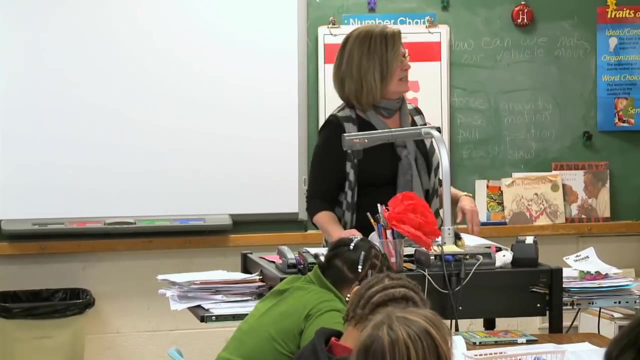 Okay, Okay, Okay, Then you're observing, You're watching and you're recording what you're observing. You're going to do that with 2 small washers, 4 small washers, 8 small washers, 16 small. 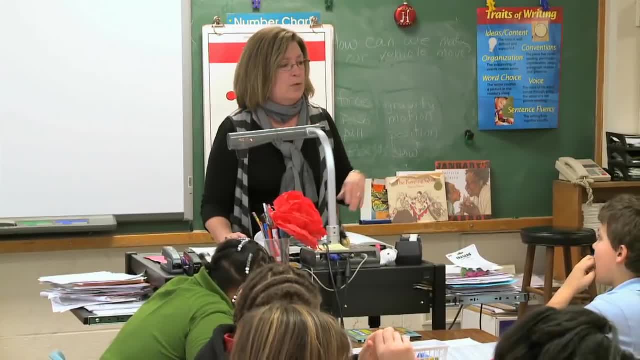 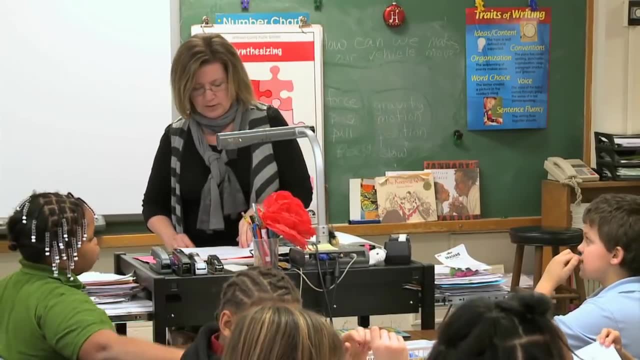 washers. or if you don't want to use 16 small washers, you use 1 large washer. Okay, And each one of you has one of those. Once you have done your washing, you're going to do the same thing. 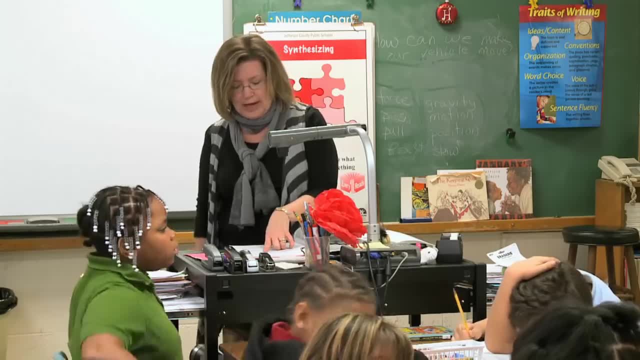 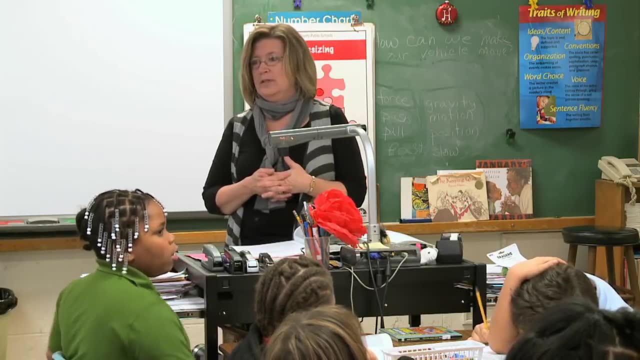 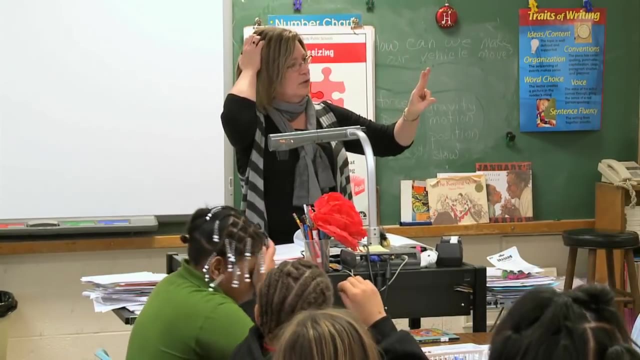 Once you have done your observations, then you're going to rank the speed. You're going to look and see which one was the slowest And you're going to give it a number value of 1.. Your next slowest is 2 on up to 5.. 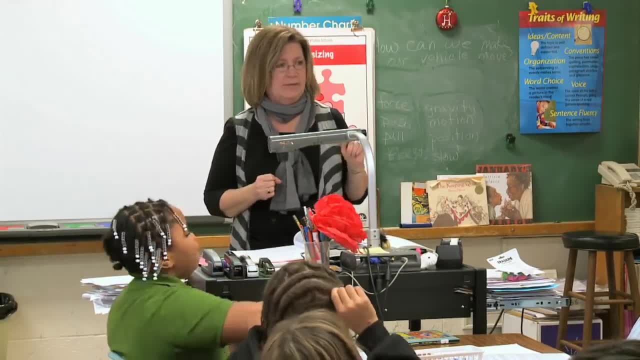 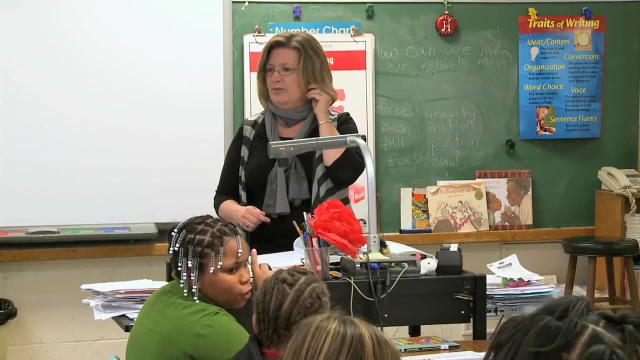 What number's going to be your fastest? 5. 5.. So each one will have a different number, from 1 to 5.. Your slowest To your fastest. Okay, We're going to start with the reading of the instructions. 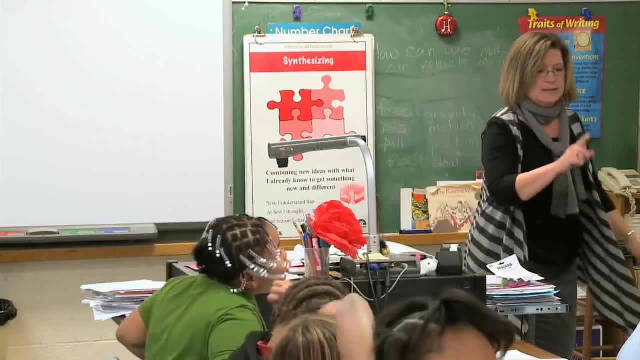 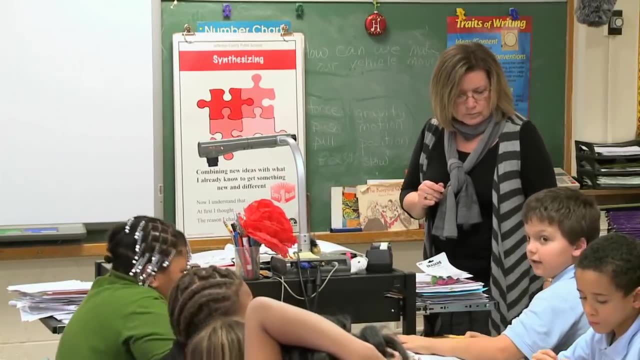 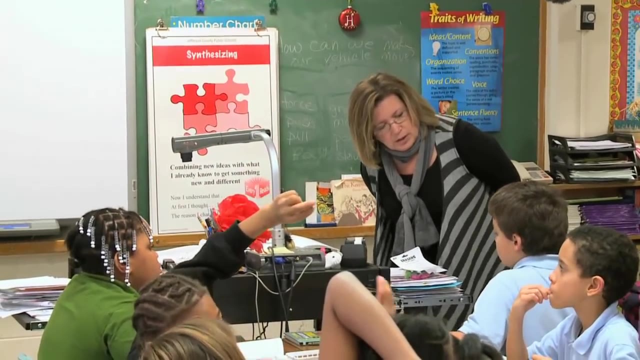 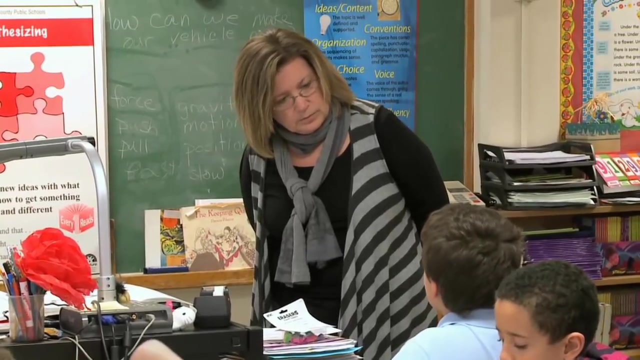 Please turn back to page 13.. Yes, When we're doing the rankings it goes. Let's listen. It might be your question: If it goes a certain speed and then half of that speed, Can we like 1, 1⁄2,? can we like put 1 and then the fraction 1 1⁄2?? 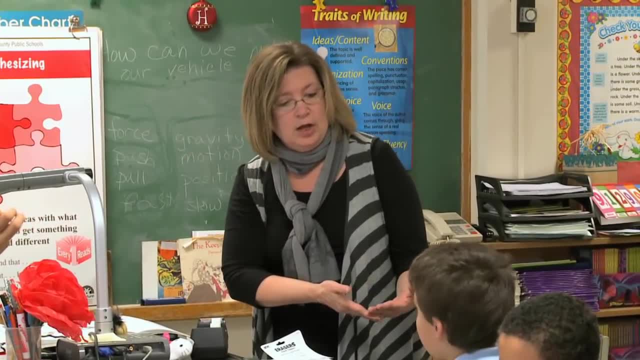 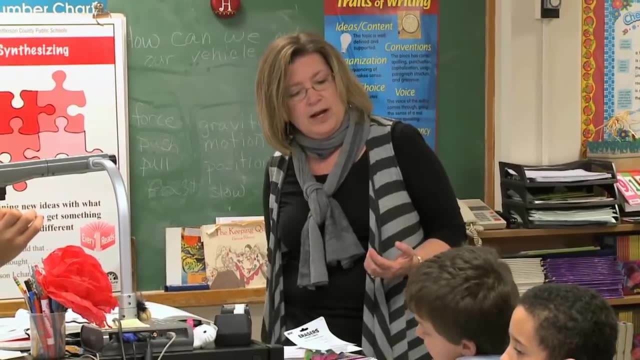 Well, you're not going to rank them until you've looked at all of them. Okay, Until you've done all the testing, And then it's only going to be 1,, 2,, 3,, 4, 5.. 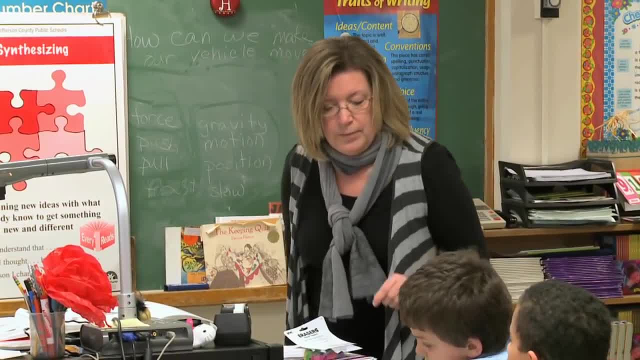 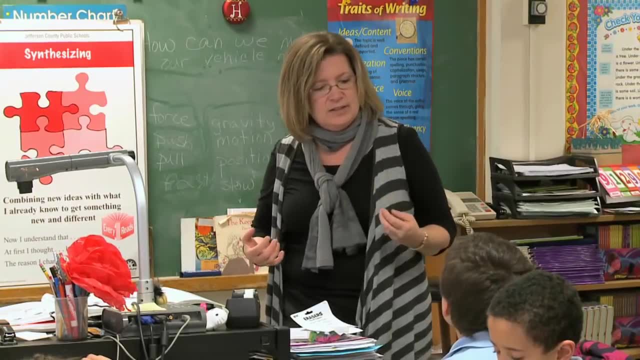 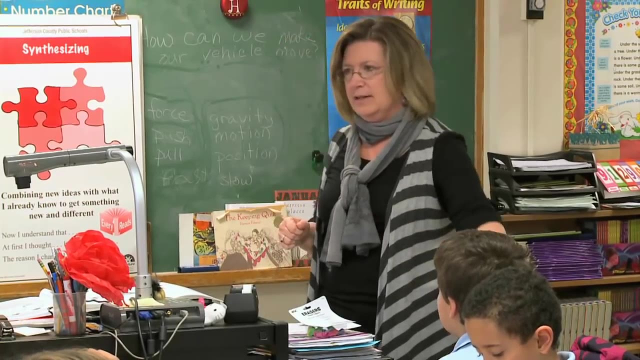 Okay, You can state that 4 small washers went twice as fast or twice as slow as 2 small washers. Okay, And that would be part of your observation. That's what you're writing down. That's an excellent question. 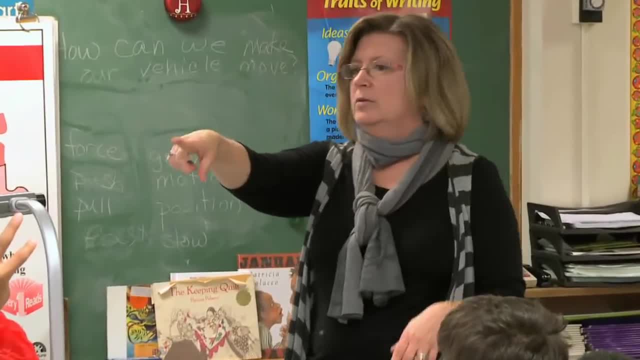 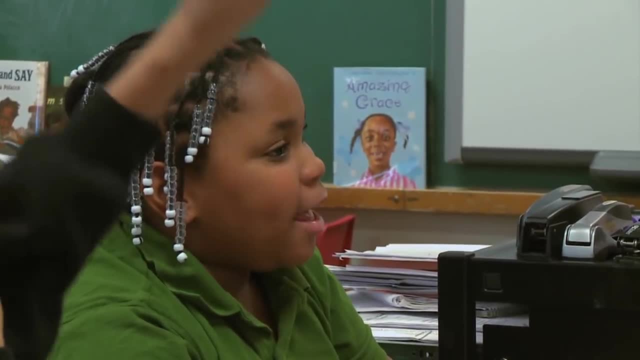 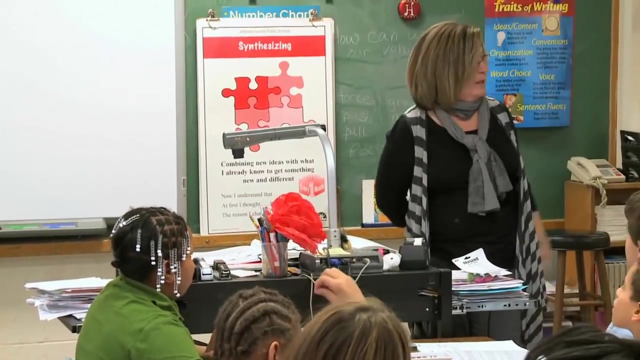 Another question: No, Yes, No, you're fine Me. Uh-huh. What happens if, like, the car falls because of the two washers on it? Well then, you just pick it back up and put it back up there. 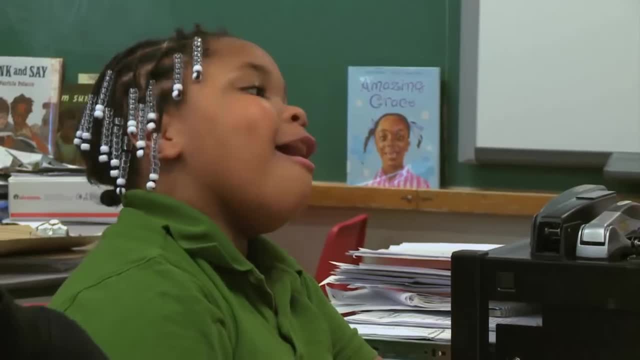 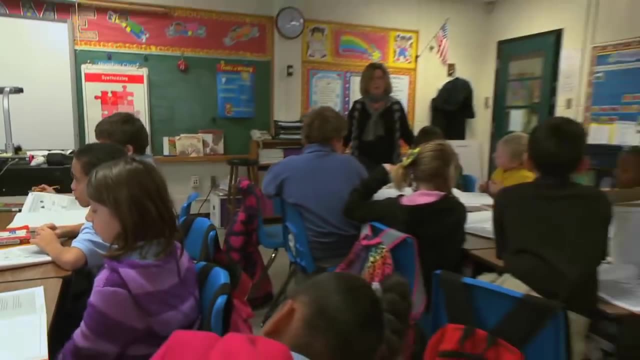 If the car falls, it falls Okay, that's okay. All right, Sit down And I'm going to give you a few minutes to read. You all can take turns reading instructions And let's go Each group, Okay. 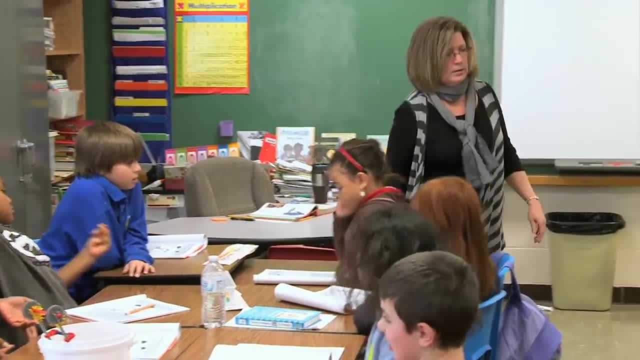 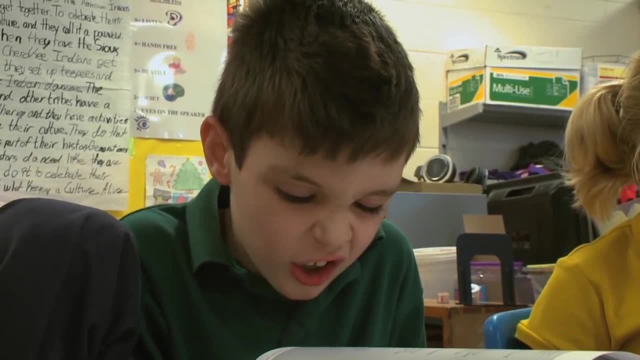 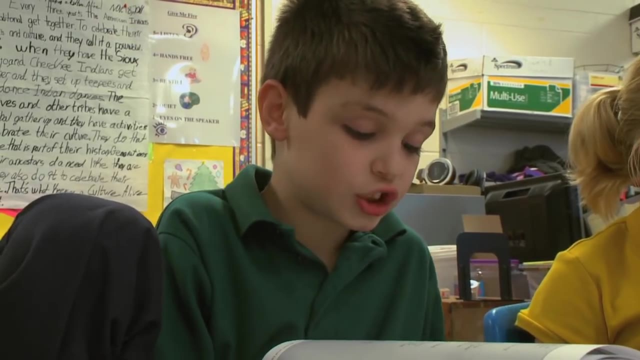 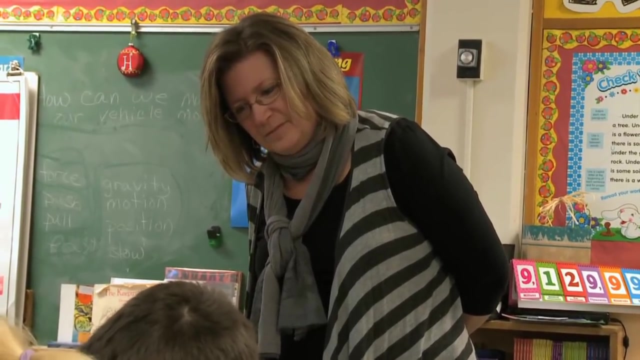 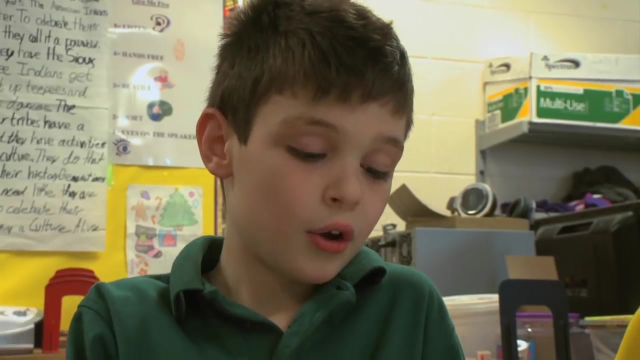 No, No, I said you don't leave until this is done. Okay, All right. I can't pronounce it by Assigning each triangle number from 1 to 5. Trial: a number from 1 to 5, with 5 being the fastest way to pull the vehicle. the fastest. 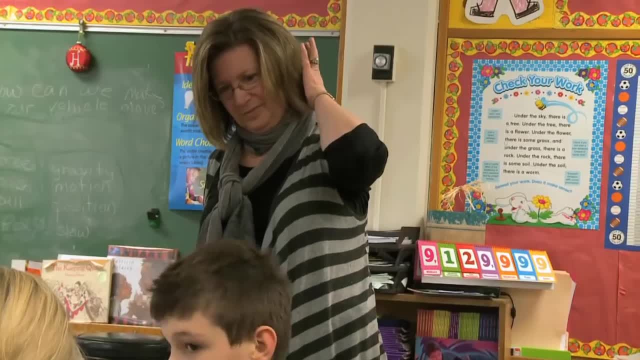 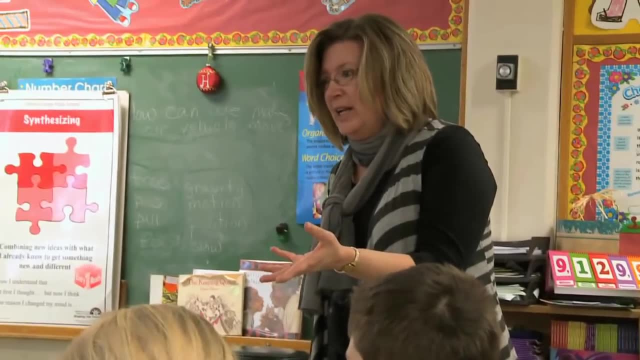 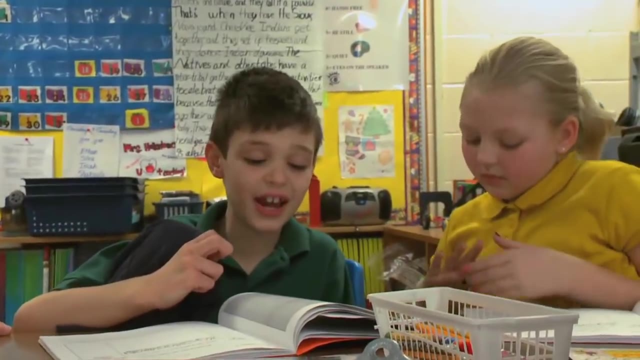 Which way pulls the vehicle the fastest? Do you guys have any questions about what you need to do? Are you ready to start? I have one more question. Okay, What's your one more question, Okay, When they say repeat the activity. 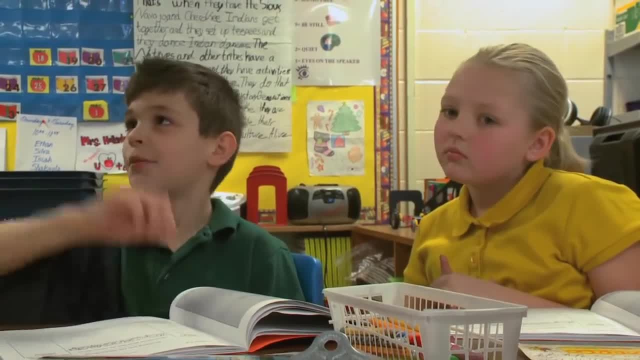 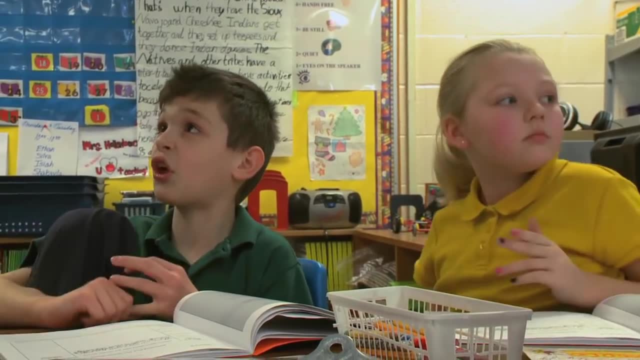 That means you do it again. Oh Okay, Okay. And when you and they were like deciding if they thought the vehicle was going to go like faster or slower, I've got my own prediction: I think it's going to go faster, but it's going to go backwards. 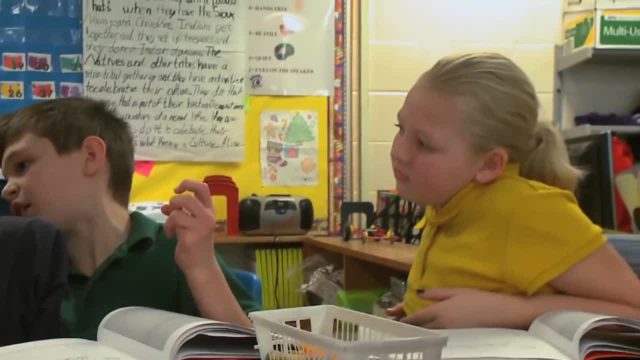 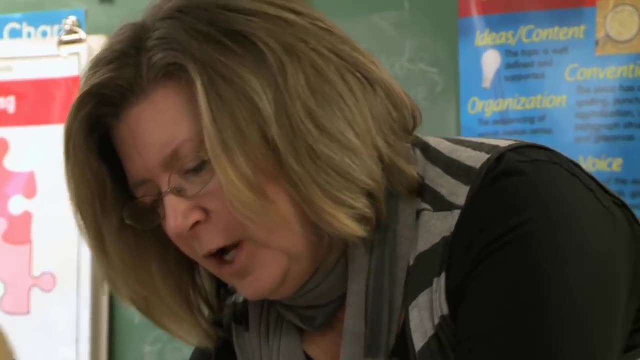 because the weight's going to be pulling it down and then the line on it's going to be pulling it forward, which is going backwards. Will you let me know how your prediction goes? okay, Now remember you're following how many of these? 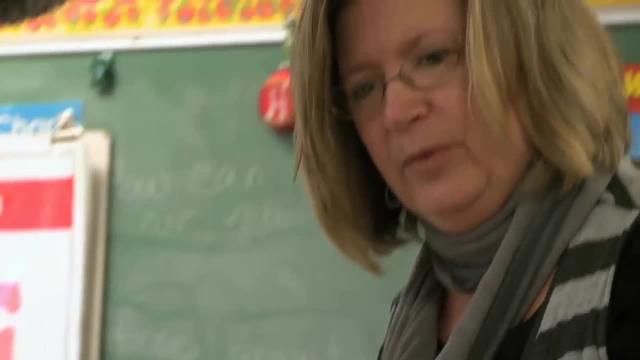 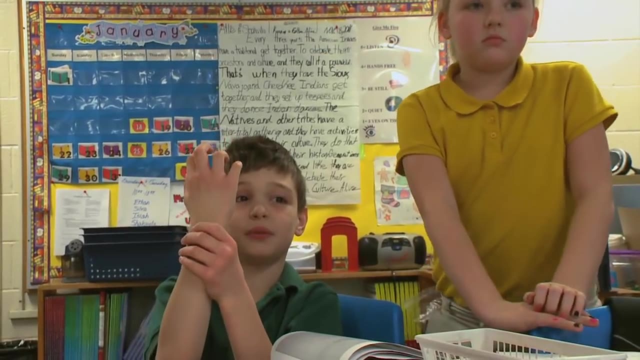 Okay, you're going to start with two. all right, You ready? I also agree with Drake, Do you agree with Drake? Yeah, because the weight's pulling it 16. Yeah, because the weight's It's going to go faster than all of them. 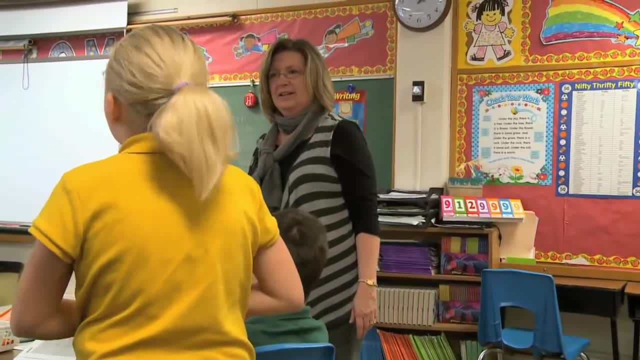 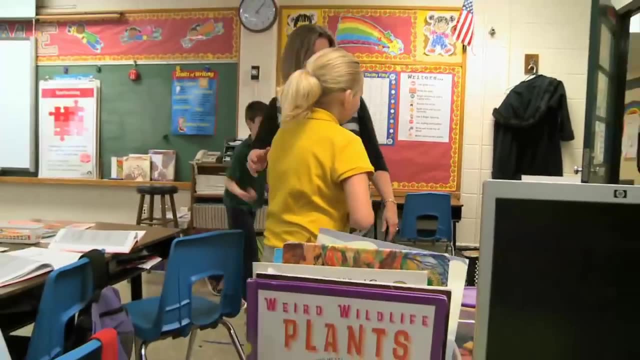 Yeah, okay, It's probably going to go off the table, All right, Well, let's see. Not yet, not yet. Okay, Let's start. Okay, Okay, Okay. have you guys finished your reading? Yes, Do you think you're ready? 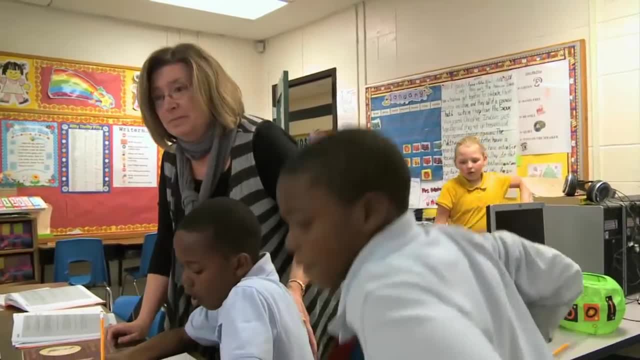 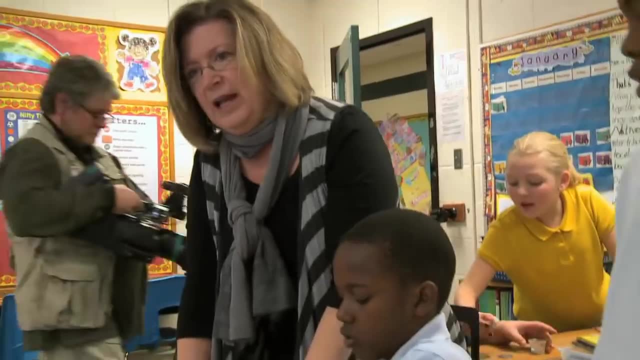 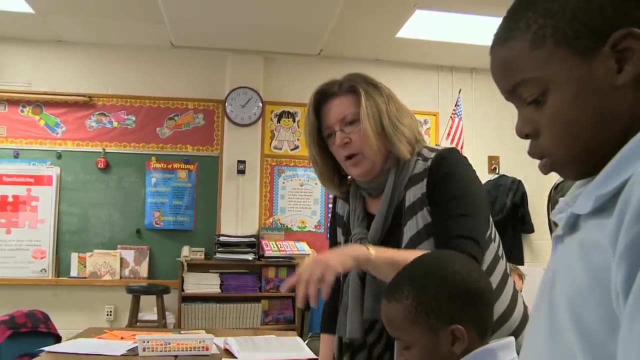 Yes, Okay, Huh, You've got four. It's okay. You're just going to put your name, okay, and I'll know what group you're in, because you're all right here, okay, Okay, now you have your supplies here and you're going to just use, use, but you're. 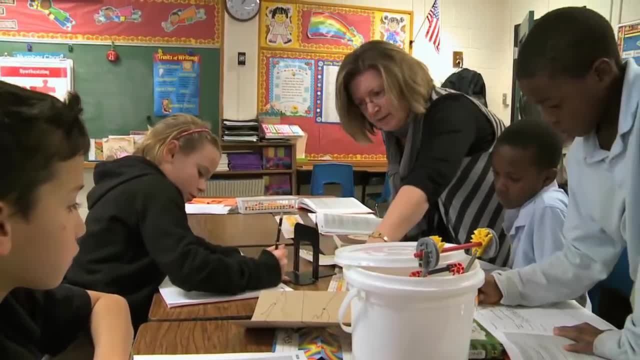 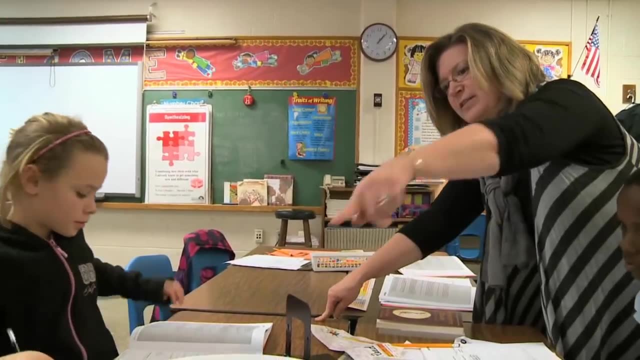 going to use, like I think your two desks are the most even, and you're going to pull these together, these three together, okay, And you're going to set it up here. This is the stuff. If you have trouble setting it up, you let me know. 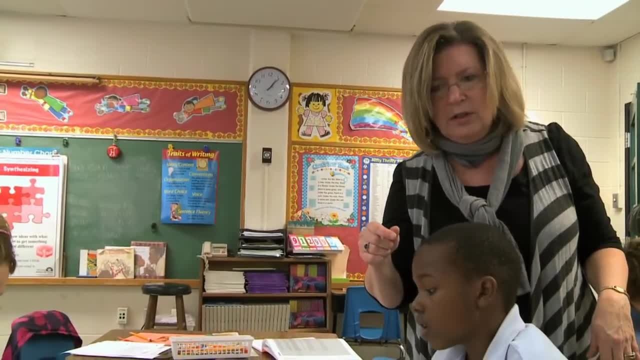 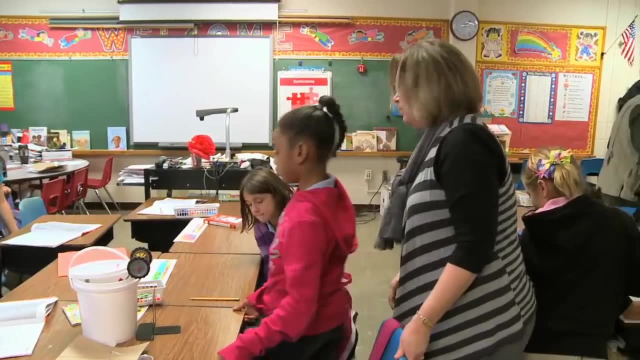 You should have. yeah, do you all have a tape measure over there too? Yes, Okay, all right. okay, I'll take this. You're going to put these together and this is going to be your. uh, this is going to. 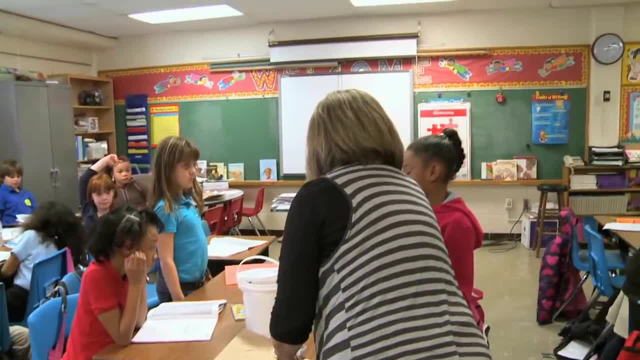 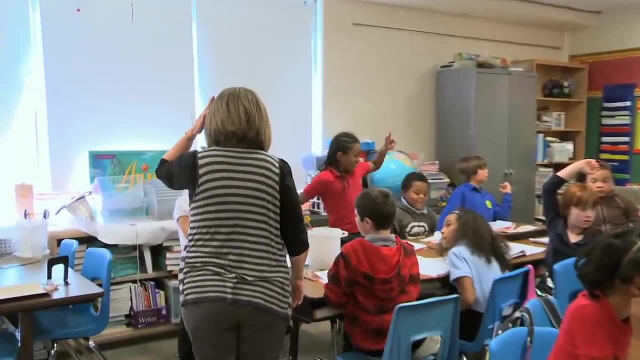 be your, your place to do your. you're going to use these three. You don't need to pull that all the way out, You just need to not have it on top of it. No, Uh, we have two. Aren't we supposed to have two? 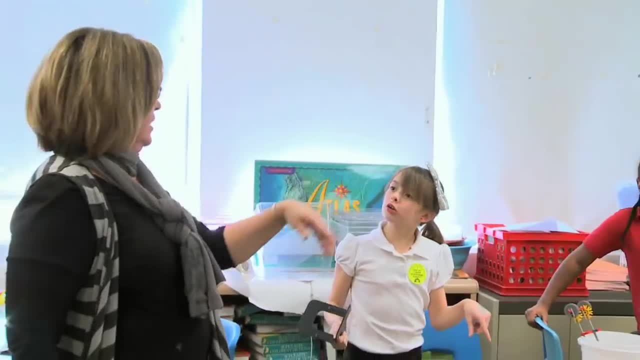 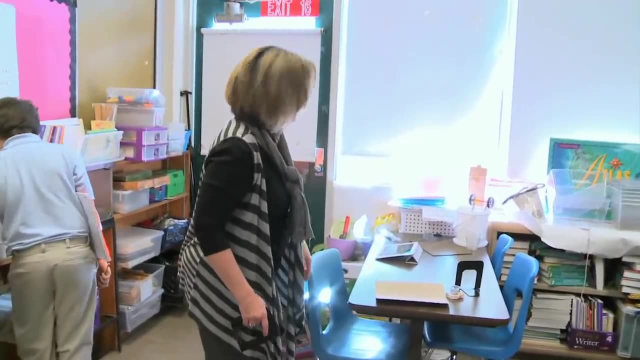 Huh, Oh, you don't need two. Okay, Can we start? Yes, you can start. You four come over here. You four are going to use this table here. Okay, We don't have a tape. We don't have a tape. 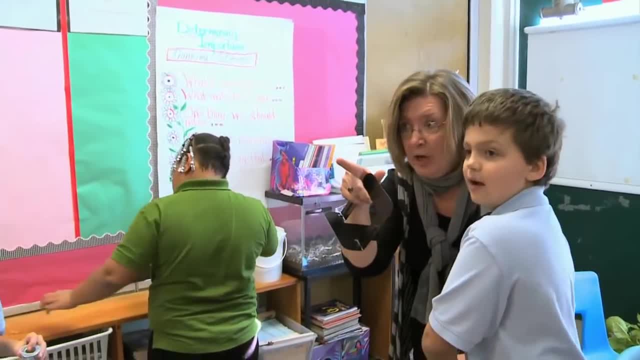 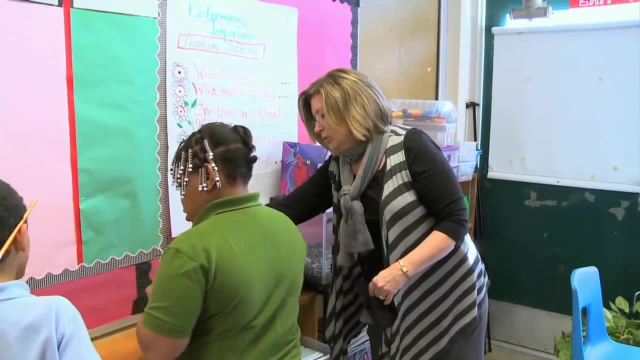 Do you need a tape measure? Look in the blue, uh, crate in one of the buckets and it's in there. okay, You're going to have to. it's got to go off this way, okay, So your, your vehicle's going to have to go face where do you think it's going to have? 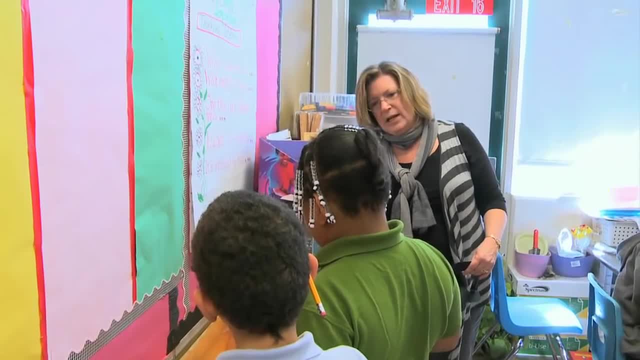 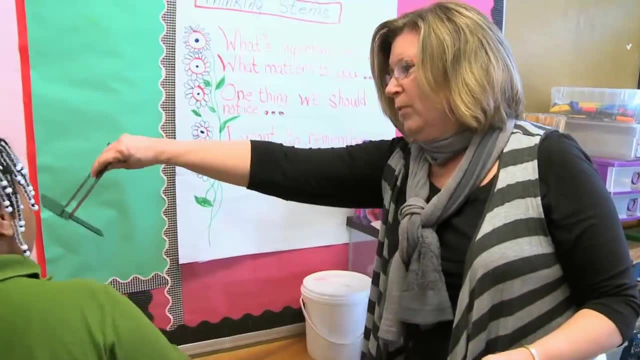 to face so that this can pull it down. Can it pull it down anywhere here? No, What are you going to have to do? There you go, There you go. So this should go where. Where should this go? There you go. 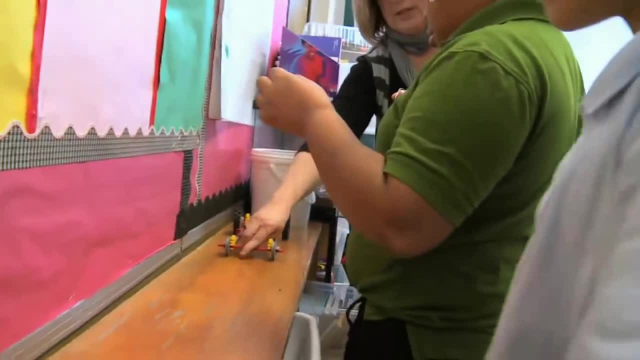 Okay, And then how does this go? You hook it onto the axle, Rick. are you done riding Two centimeters? Let me see if you're done. Okay, It moved a little bit. Okay, And it moved 15 centimeters. 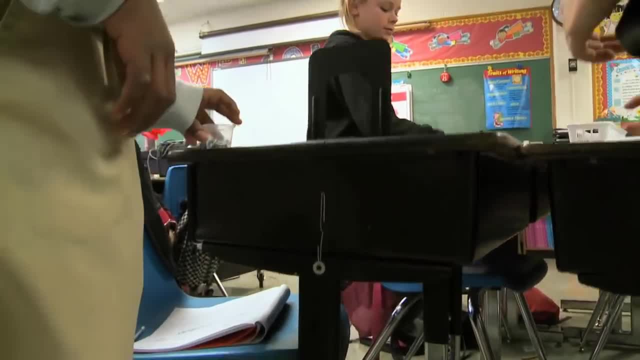 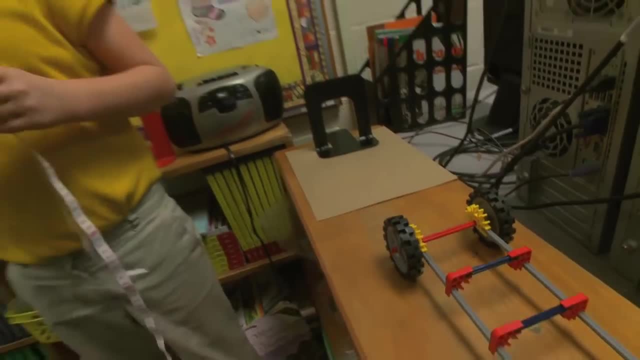 Right Press it. Okay, Where do I put it? Where do I put it again? You need two more. Yes, Yeah, Two more. Let's do six feet. Let's do six feet. Two more, Two more, Two more. 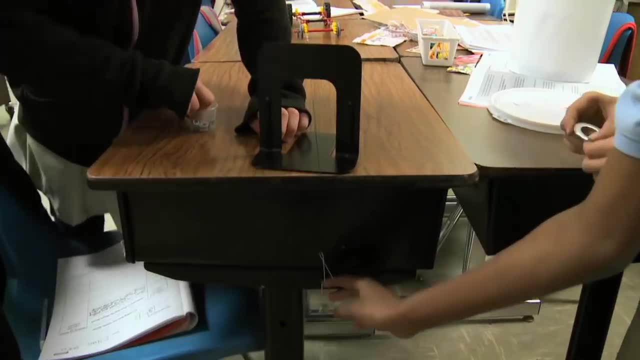 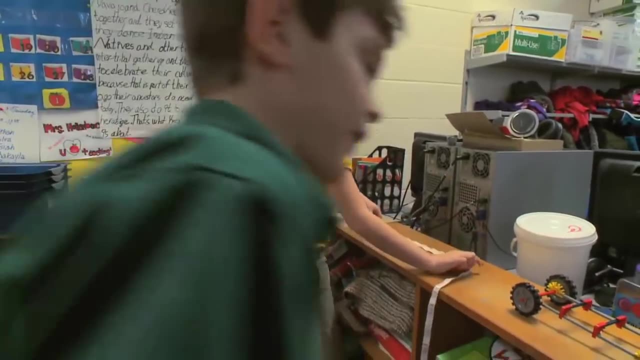 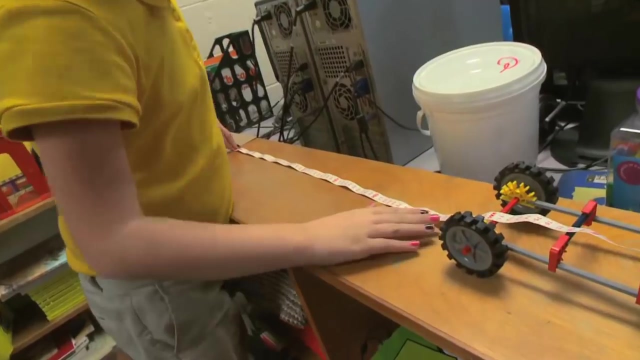 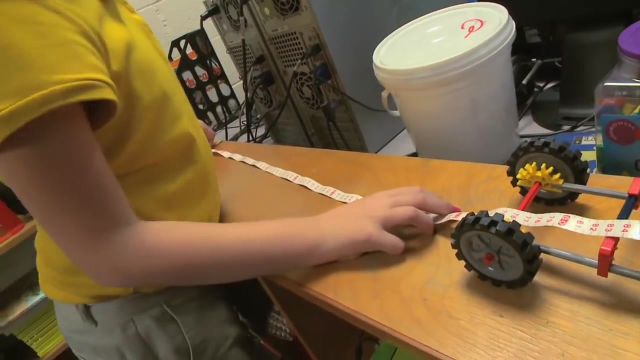 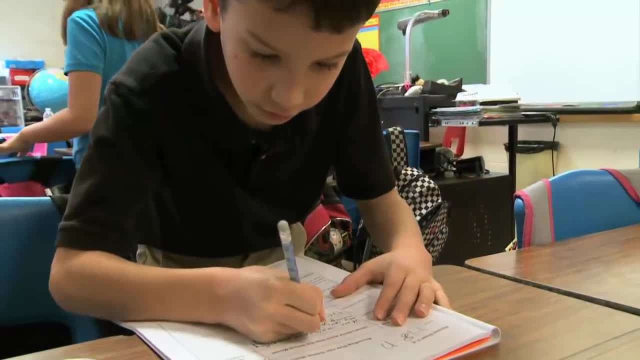 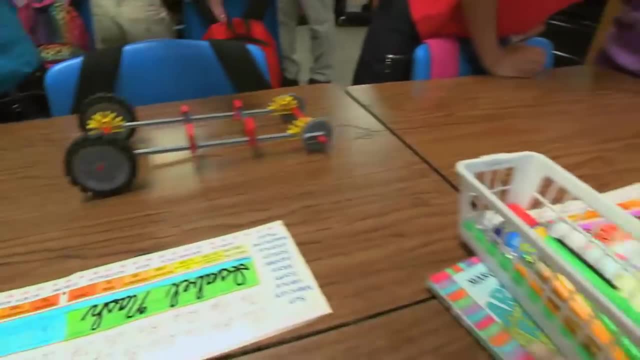 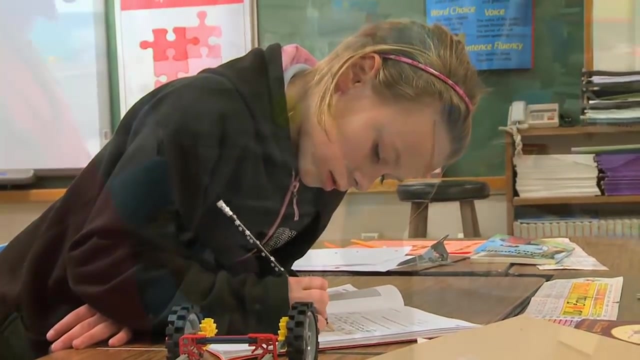 What About 60,, 69., 69. I like the way some are recording what they saw. Excellent, Thanks everyone. Thanks everyone. Did you record what you saw? Okay, now, I got it. Now look. 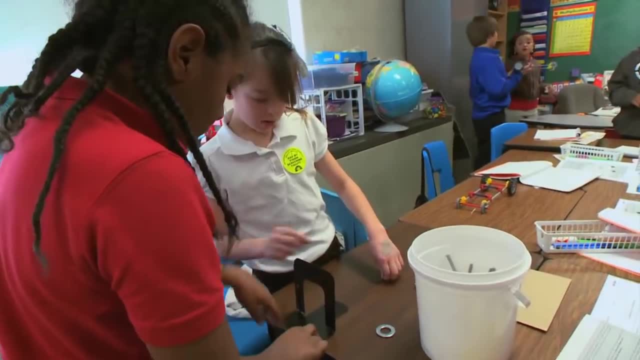 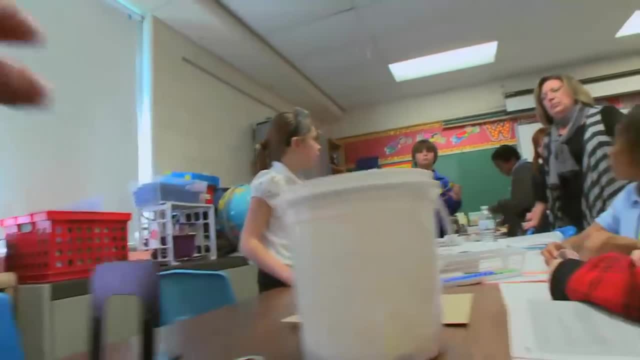 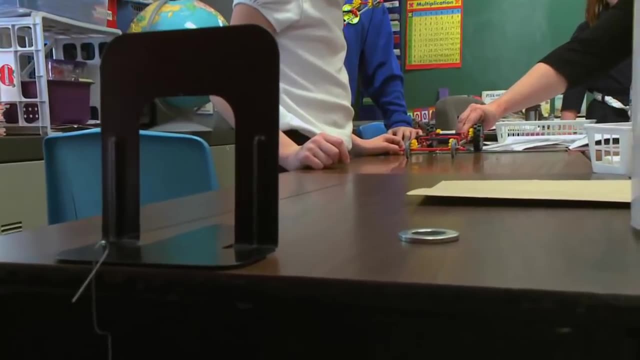 Pull it back all the way up again. Let it go. Okay, let's try it again. All right, Now, wait a minute, Hold there. Okay, Let it go. One, two, three, Let it rip. Oh, that's good. 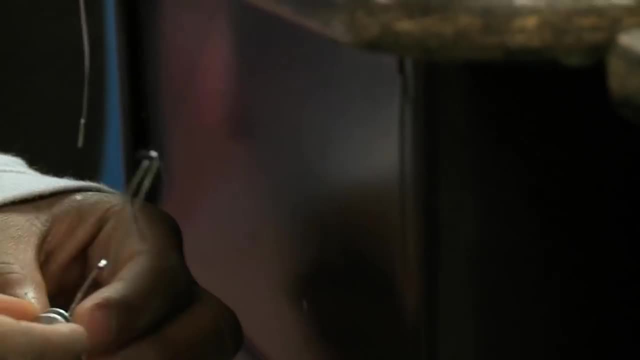 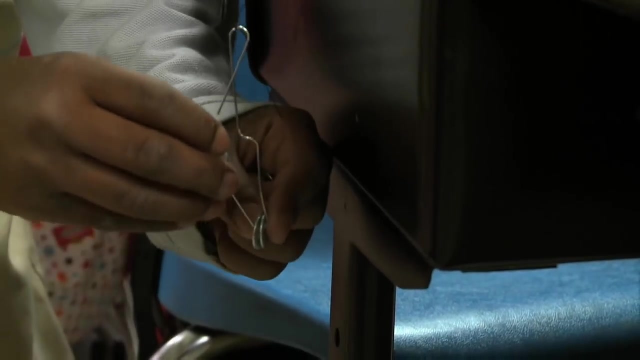 Okay, It didn't go nowhere, All right. All right, Then you can write that down. You can try this side if you want. Why don't you try this side? Okay, That's better. It looks like it has decimals. 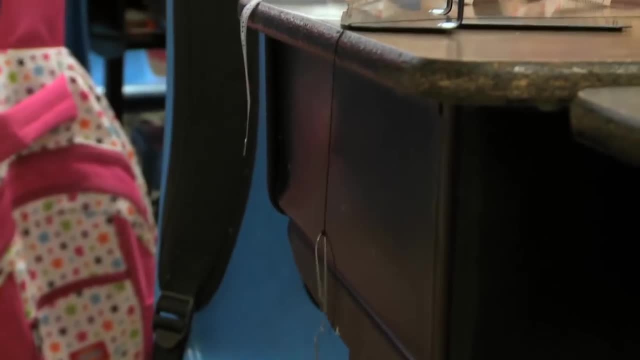 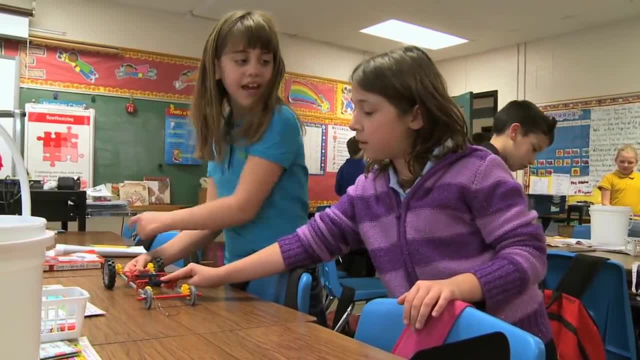 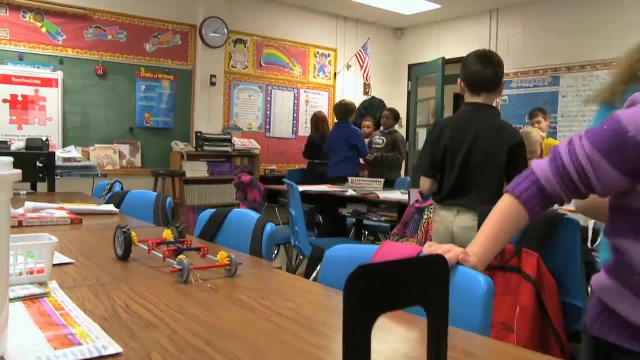 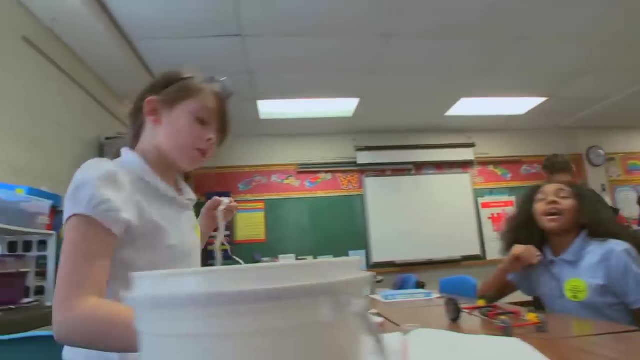 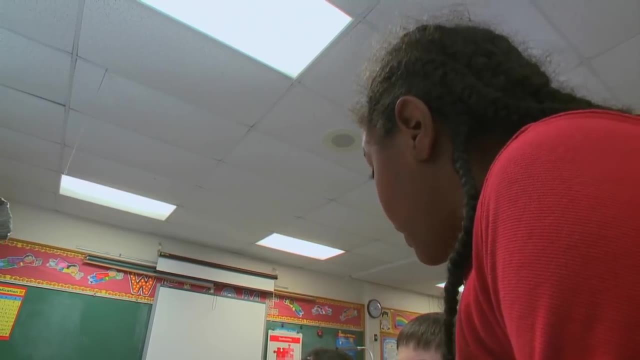 62.. No, it went in the middle, So we need to write down our response. But don't put the speed there. No, we don't. We have to wait until we have a right to speed and we're going to see what's going on. 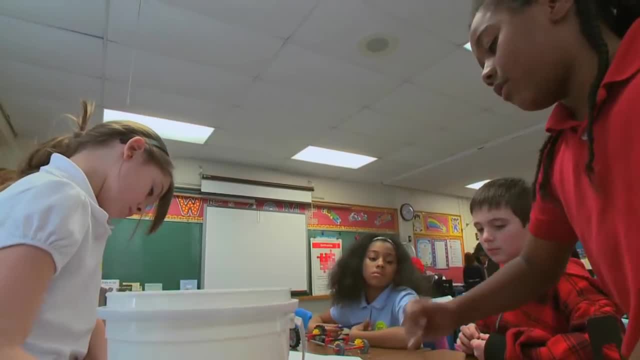 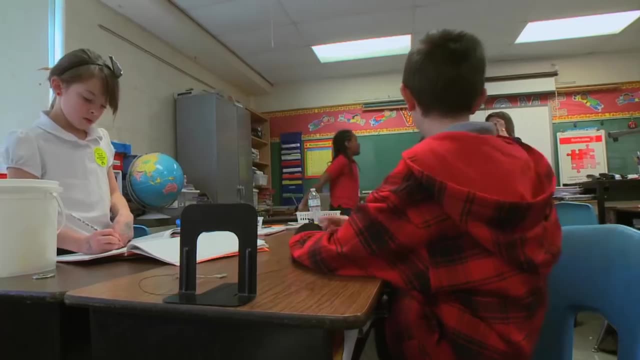 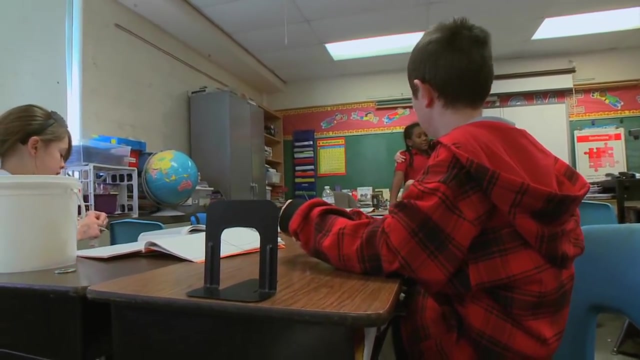 Okay, Whichever one goes slowest and whichever one goes slowest. one of them wants to go the fastest. We write our responses first. What technical difficulties are you having? Don't we have to write the speed after we do every one? 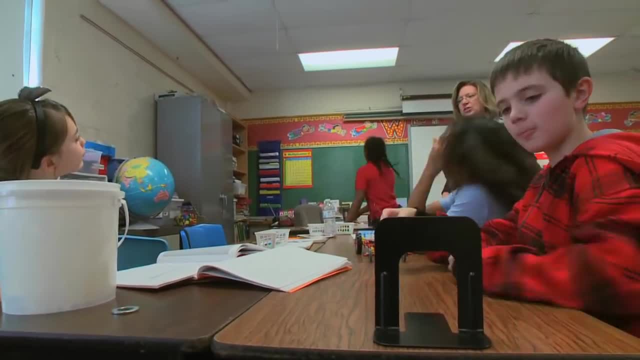 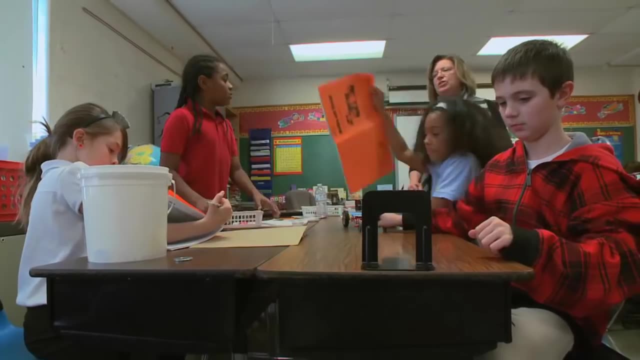 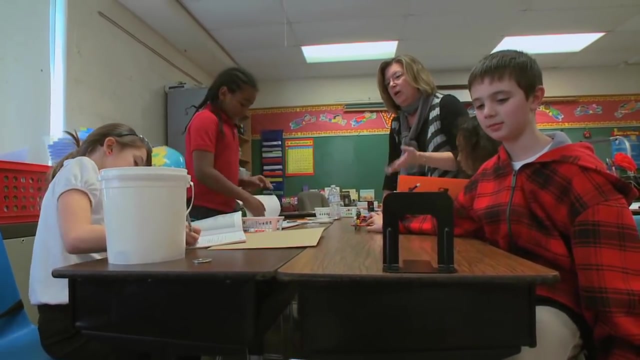 No, Each time you're supposed to write your observations, Write your observations after each one. okay, Write your observations. Do not do the speed. Okay, Erase the speed. No, you can't do that until you've written all your observations. 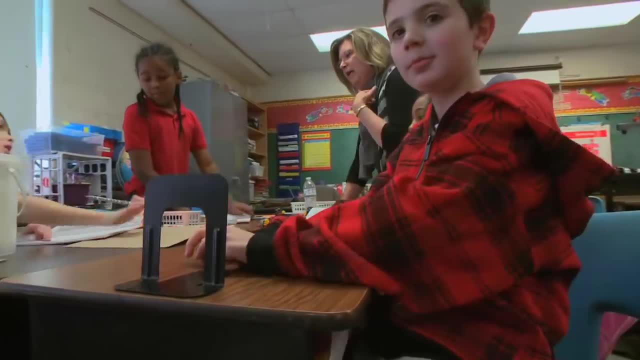 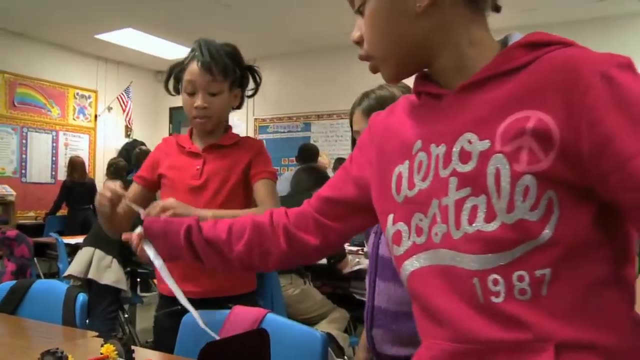 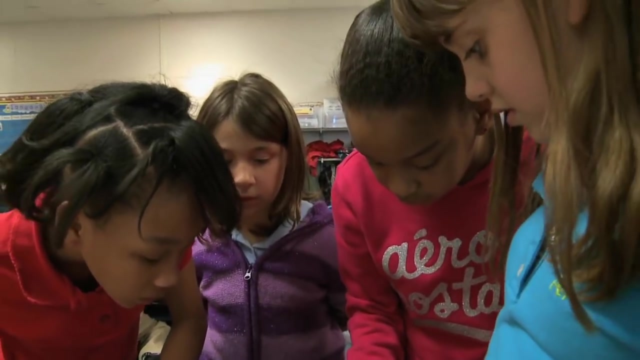 Okay, I believe that was in my directions. It was in these directions that you read: We didn't get it all the way right. there It's a this, It's a this It's a six. No, I'm really fast. 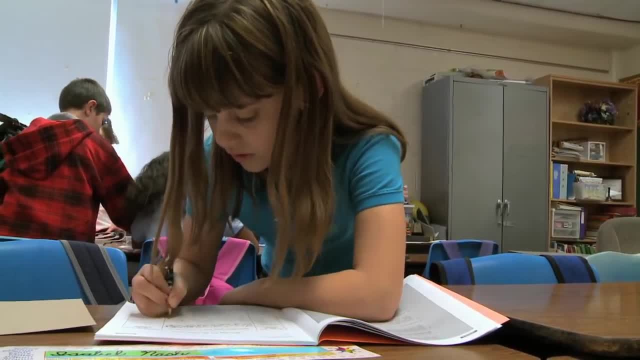 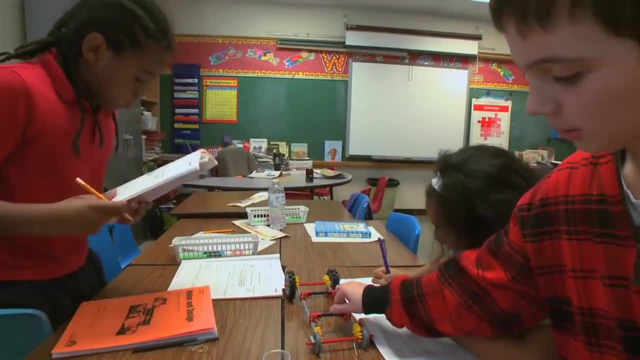 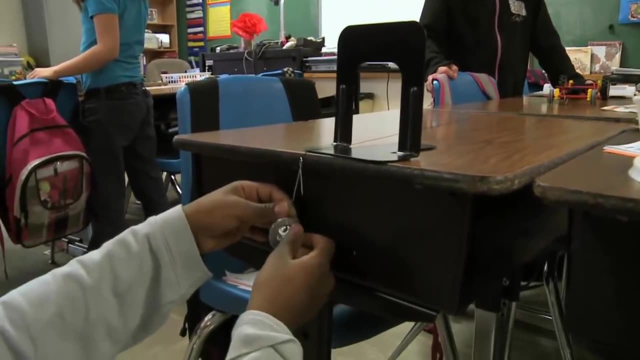 I didn't see it. Okay, I didn't do my observations yet, So you're going to wait a week, though, Yeah, At first, no One, Two, Three, Four, Five, Six, Seven, Eight. 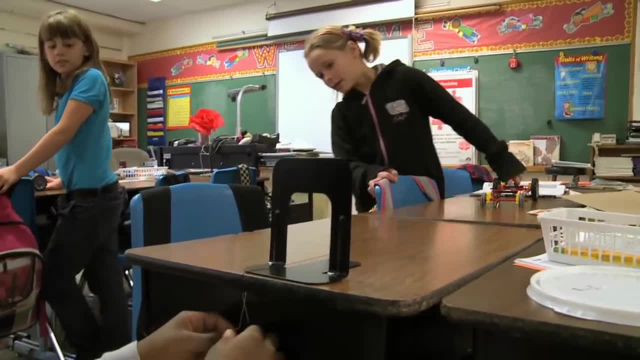 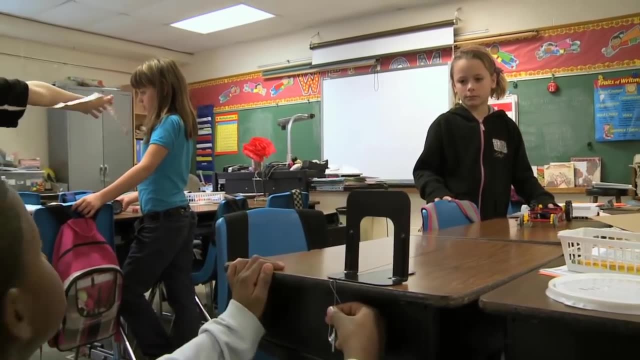 Nine, Ten, Eleven, Twelve, Thirteen, Thirteen, Thirteen, Twenty, Twenty. That's aadaki, How many seconds You can do the measuring? Uh oh, We need to Hold on. We need to have it all the way, right up to there. 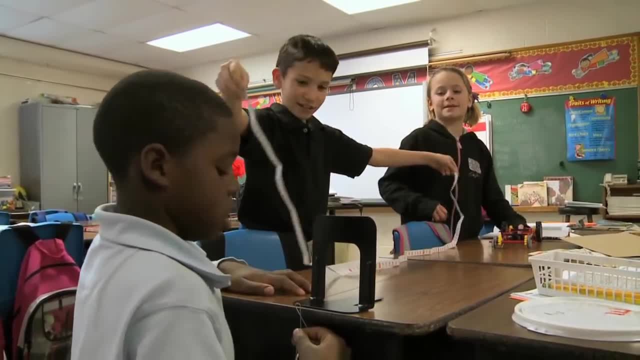 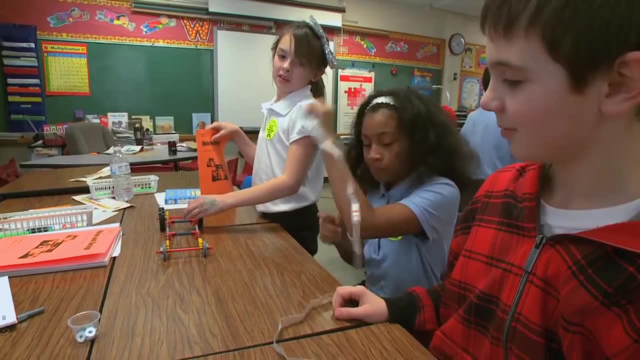 Hold, hold. Do you have this unhappy? I'm 149.. Wow Here, Good job, Hold on, We need to measure it. Oh, it's a measuring. Do we want theUNI? Yes, Okay, two. 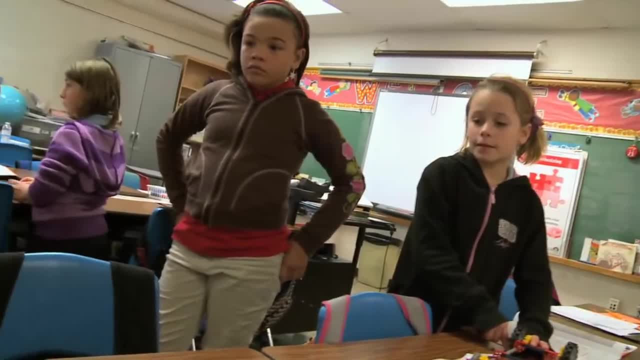 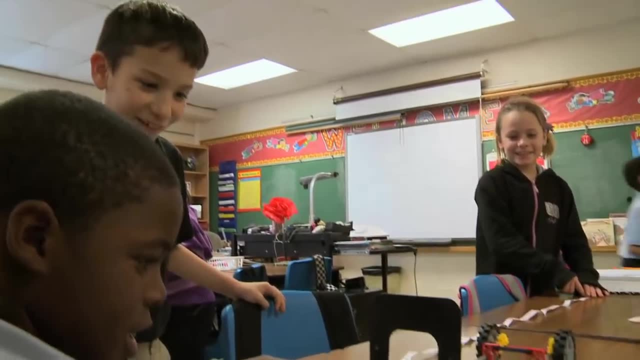 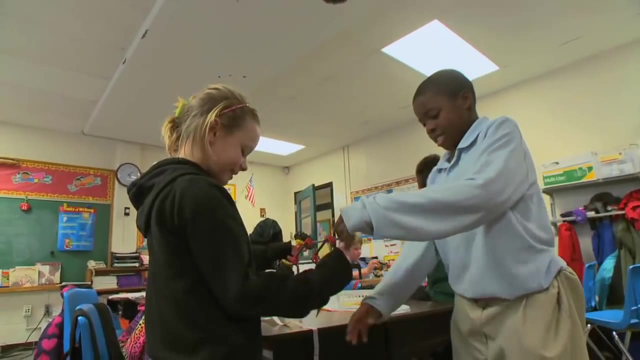 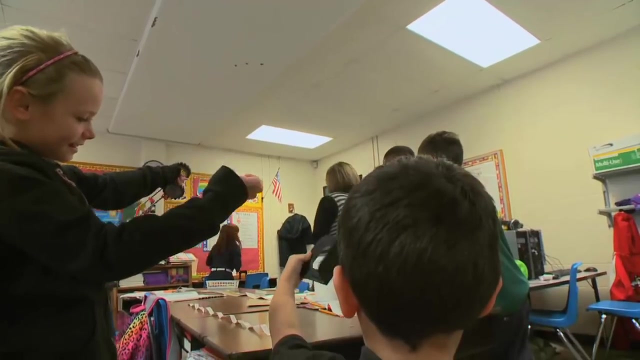 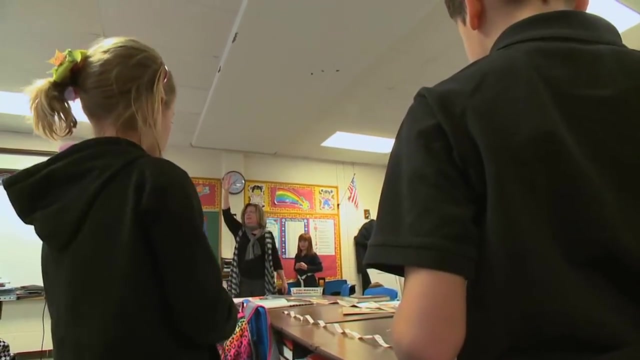 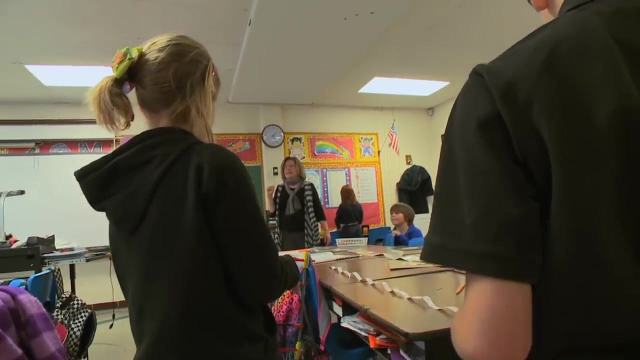 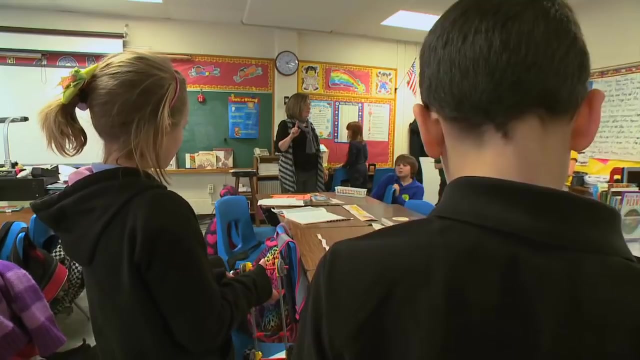 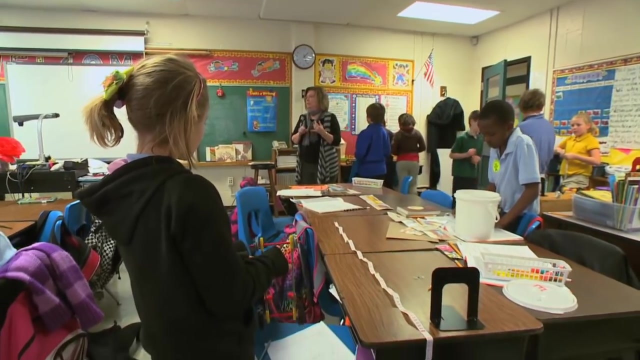 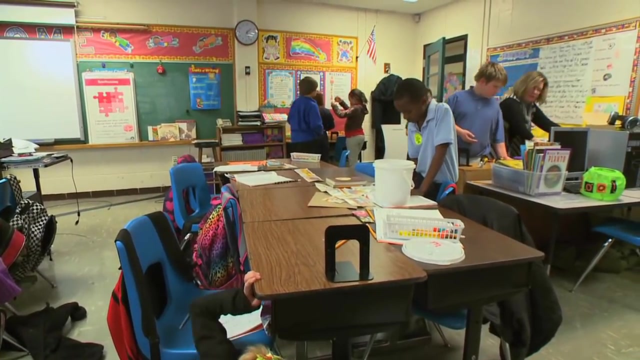 One, Two, Three, One, Two, Two, Three, four, three, two, one freeze. okay, listen to all instructions carefully. when I say go on a voice, you are going to put the tape in your bucket, your vehicle in your bucket. you're going to take the cardboard that you got and the 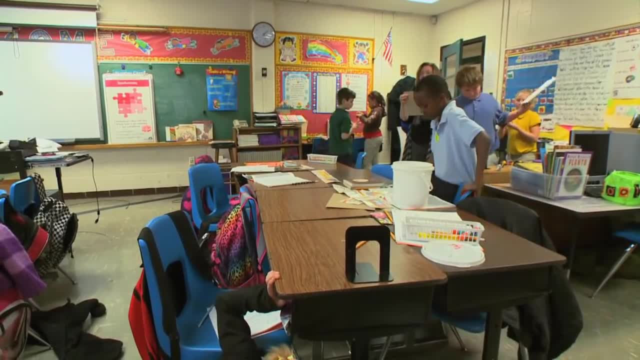 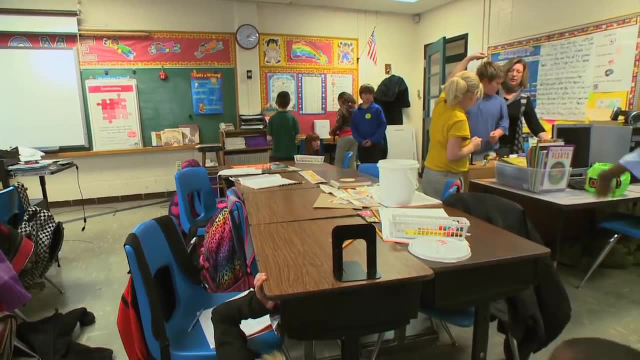 string and you're going to wrap it back around so it does not get knotted. okay, and you're going to put the tape in your bucket and you're going to take the tape and you're going to sit your bucket with your vehicle and your cup of. 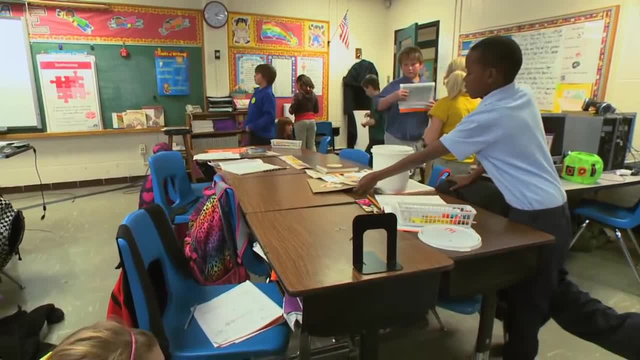 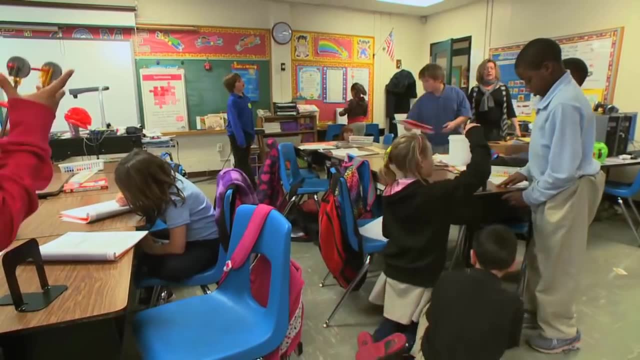 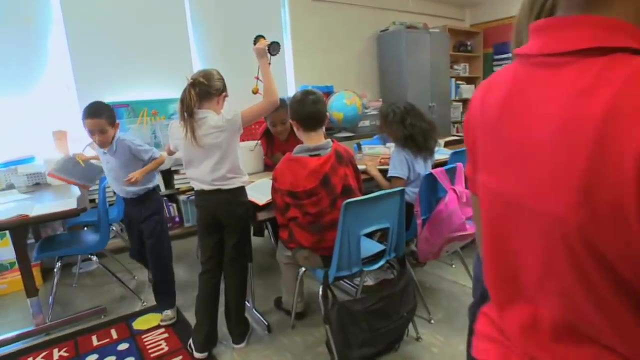 your cup of washers. well, I just spilled it, your cup of washers, with your equipment, without doing what I did, spilling it all over the place. now, those who have their buckets at the tape, listen, I did not say go. did you hear me say go? no, the ones that have their buckets. 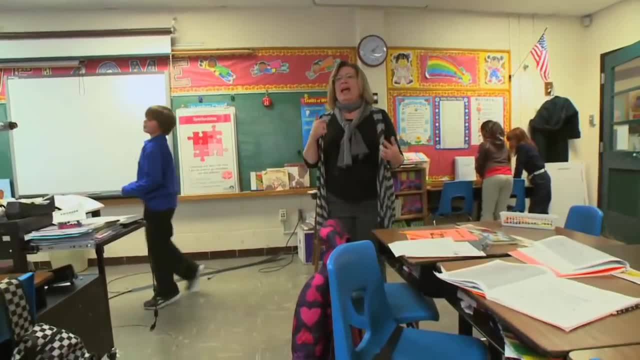 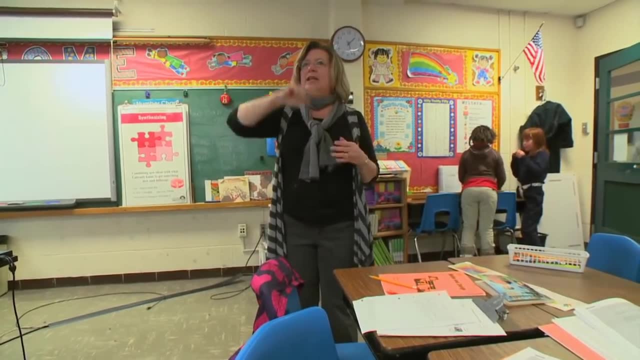 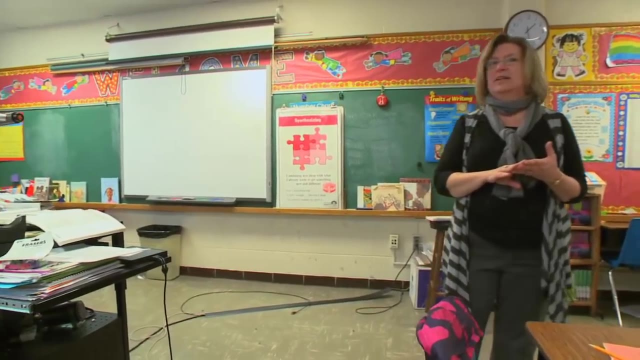 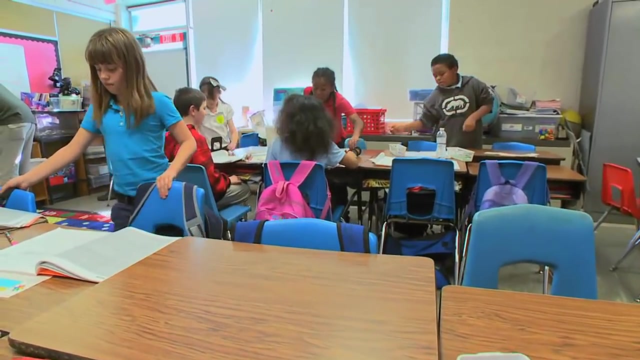 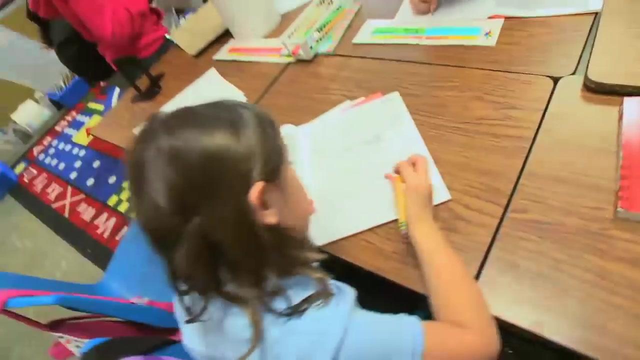 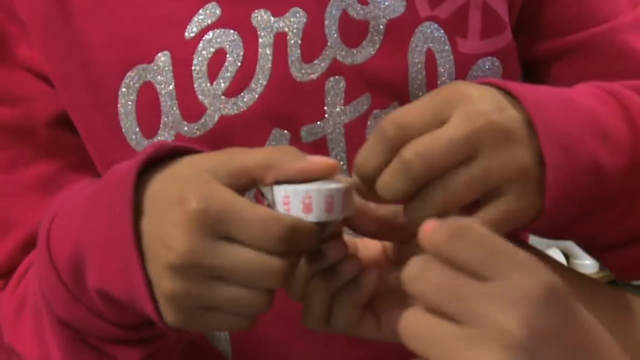 on the table when you have your equipment together. you're going to take your equipment, put it together on the back table over there. go you. I'm seeing some good cleanup over here working together well.